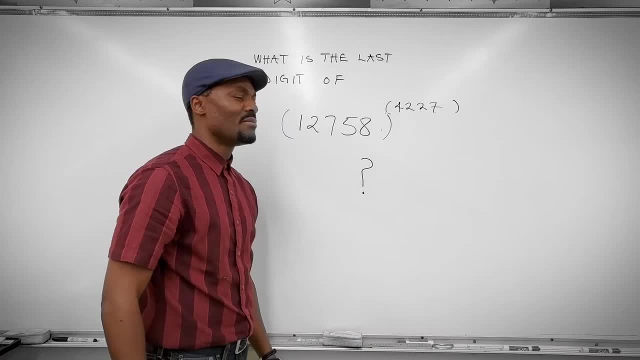 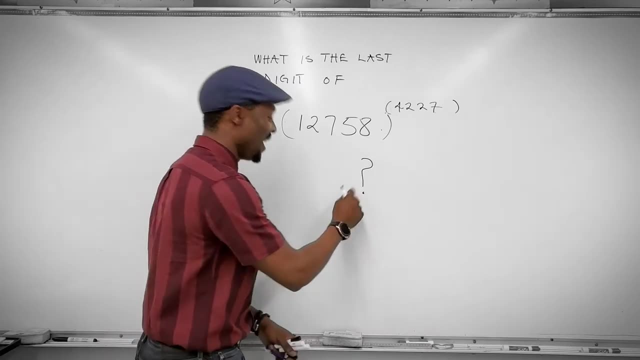 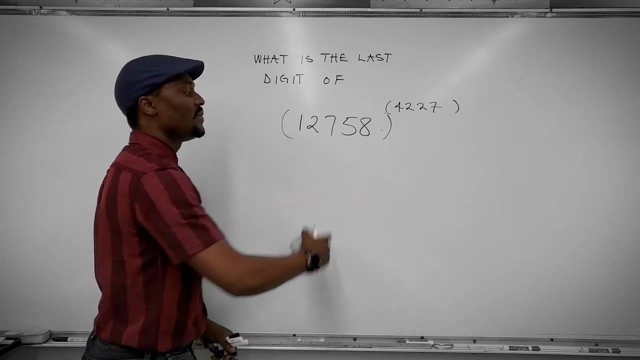 need a grand computer to do this. Maybe I could put that in my computer. Your calculator will fail, Okay, so don't try it. Don't try this at home. Okay, let's go to the question. So this is the problem we're trying to solve. It's 1,000, 12,758 raised to the power of 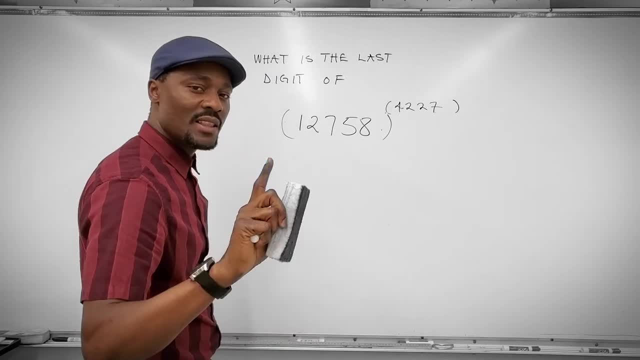 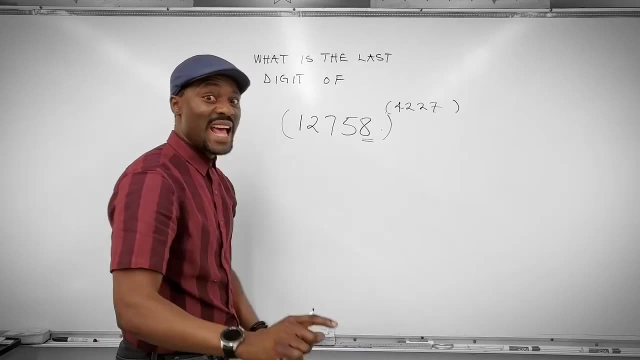 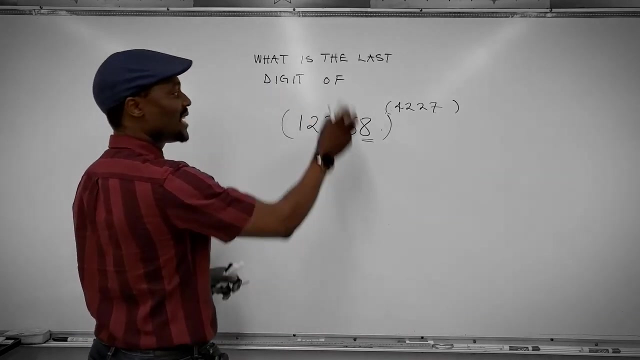 4,227.. What's the last digit? There's only one secret: The secret to this problem is the last digit, The last digit. So this is the last digit problem. It is not the last problem. Let's go on. Okay, I'm going to take this out. I'm going to write the question. 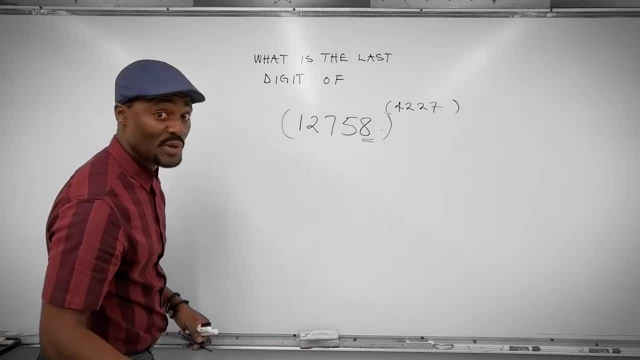 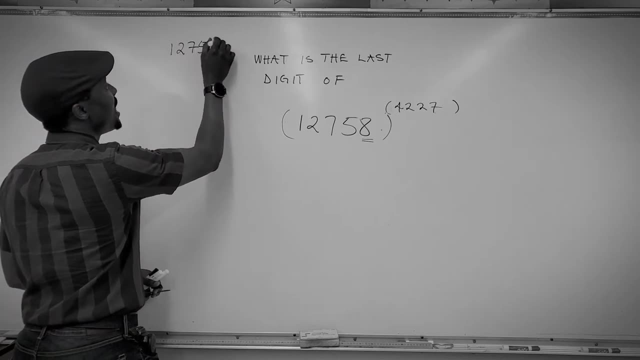 here so we can always come back to it. We've got to know what problem we created. When you create a problem, you better track it. Okay, so we go 1,, 2,, 7,, 5, 8 to the power. 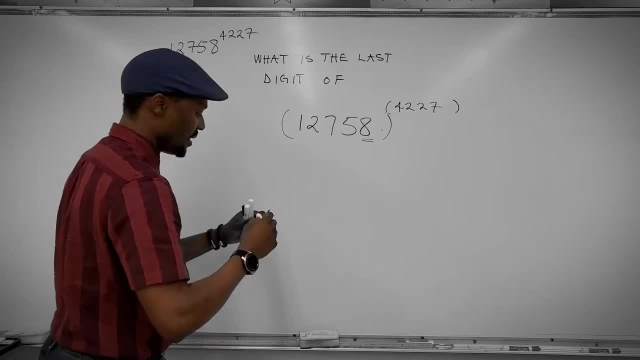 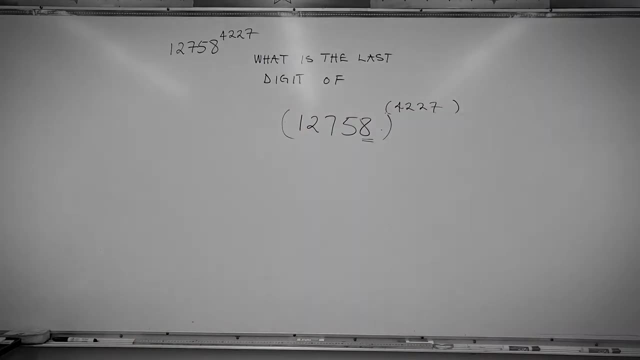 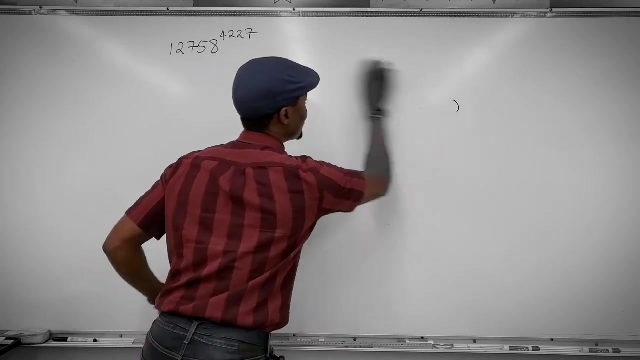 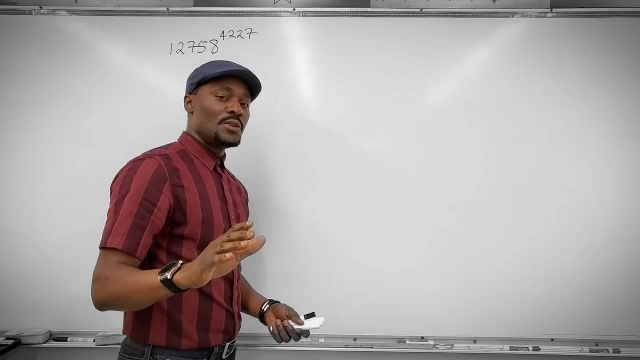 of 4,227.. I'm getting rid of this. Let's get rid of the problem for now. The problem is still there. Okay, let's go. So right now I need to explain a principle to you which I believe you may understand or may not, but if you don't, once I mention 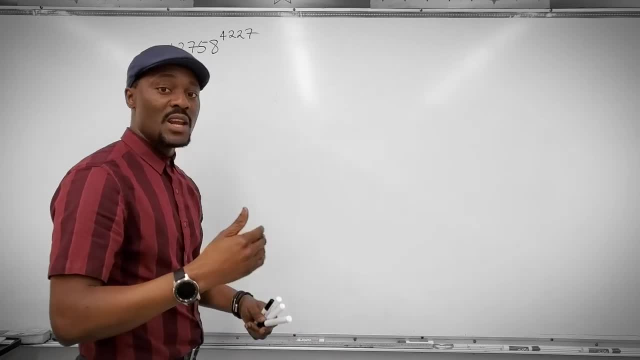 it- you will observe it- that every time you multiply a number by itself, the last digit is always the last digit. So if you multiply a number by itself, the last digit is always the last digit. So if you multiply a number by itself, the last digit is always the last. 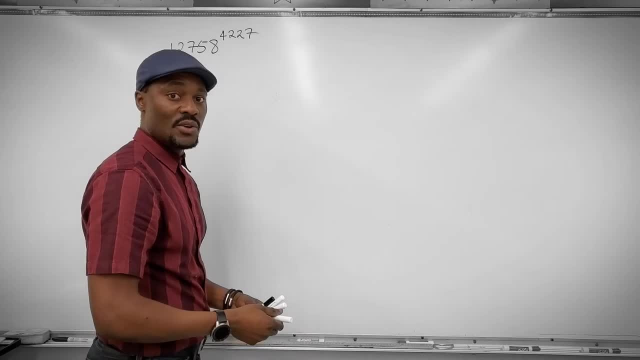 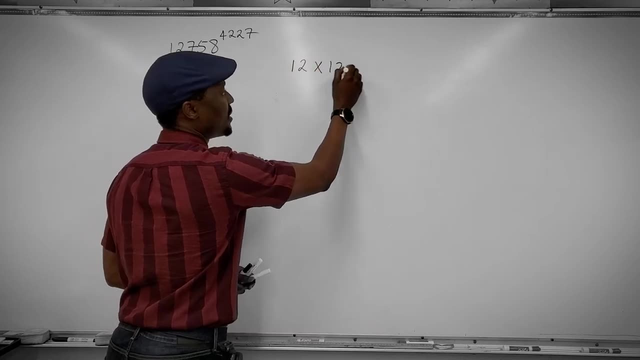 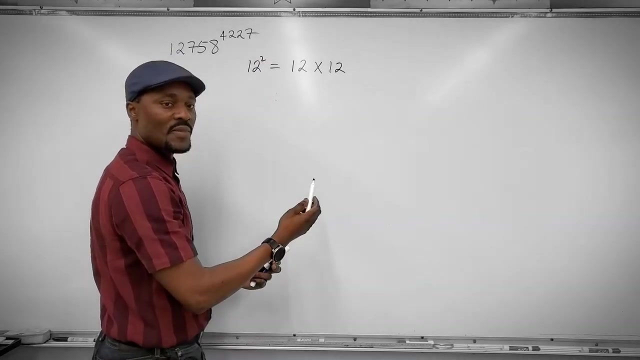 determined by the last digit of that number by itself. Okay, that's the most important number. For example, if I decide to multiply 12 by 12,, just 12 by 12, this will be 12 squared. So you get the secret. Well, the answer is 144.. But the reason the last digit is 4 is: 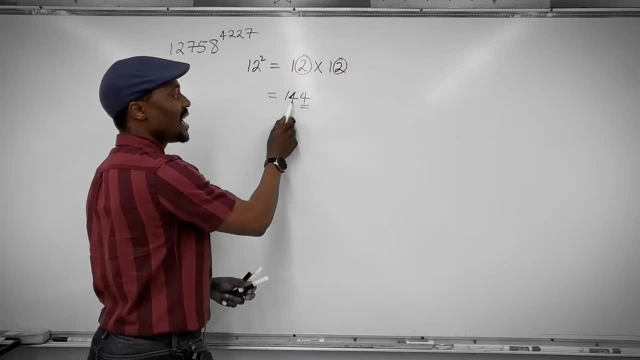 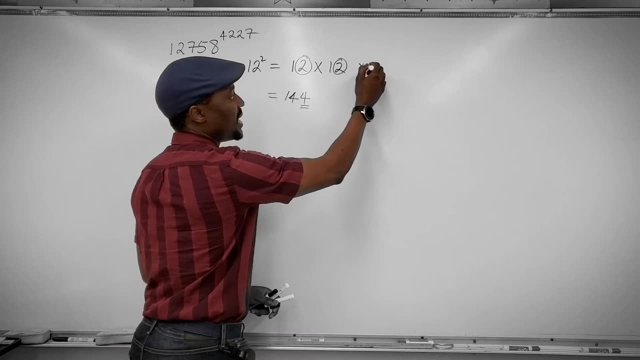 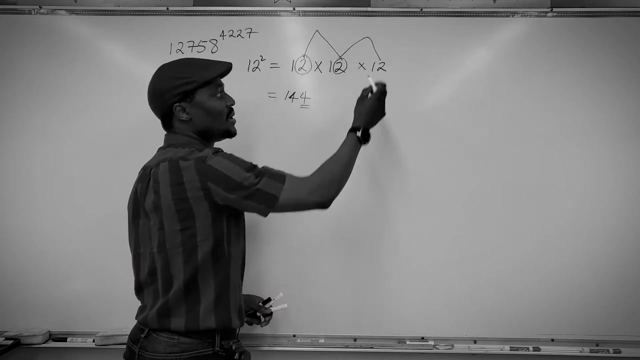 because this number multiplies this. Anything else here? Well, we don't want to do that, We don't care about that. What we care about is the last digit. And if you multiply this number again by 12, well, it's the same thing as multiplying this by 2 and then by 2, and 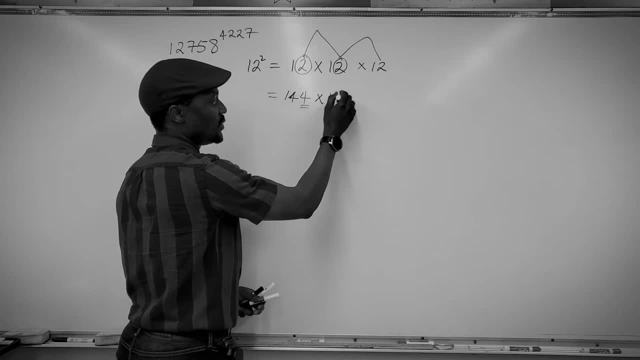 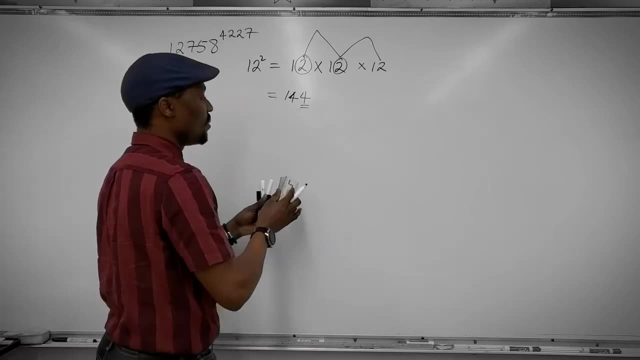 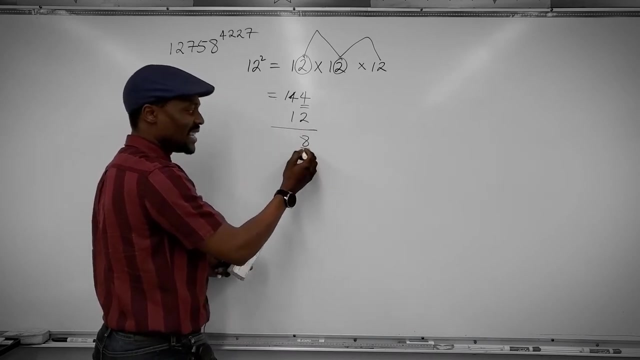 then you get 8.. So if you multiply this again by 12, the first multiplication you do is- let's say we put this here- The first multiplication you do will be 12 times 144.. Your first answer is going to be 8, your first digit, So the last digit is 8.. So if you multiply this number, 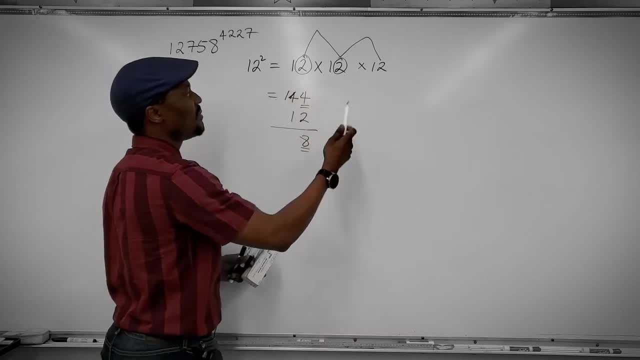 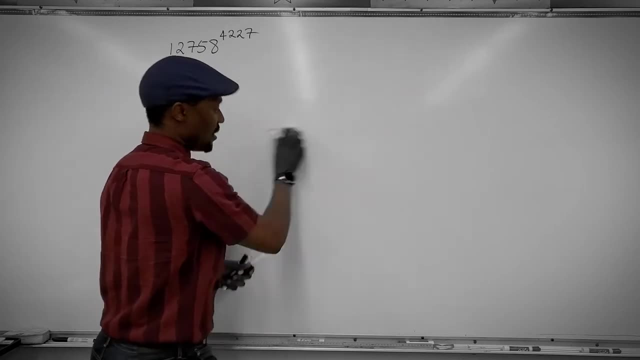 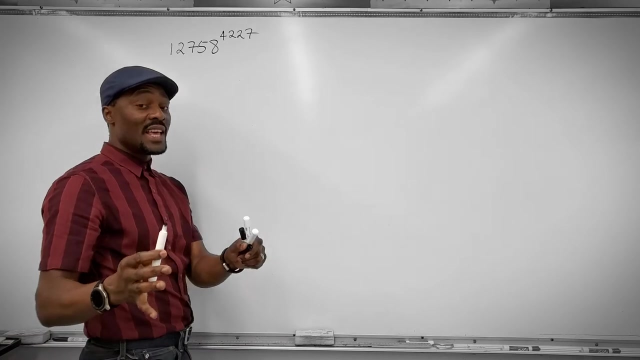 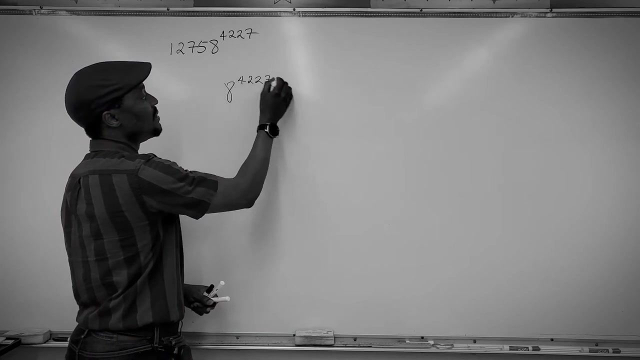 is simply just multiplying this the same number of times as you would. so the last digit of this number we have here will be the last digit of twelve thousand seven hundred and fifty eight will be the same thing as the digit you get on the end when you multiply eight by four, two, two, seven. so see this not relevant. 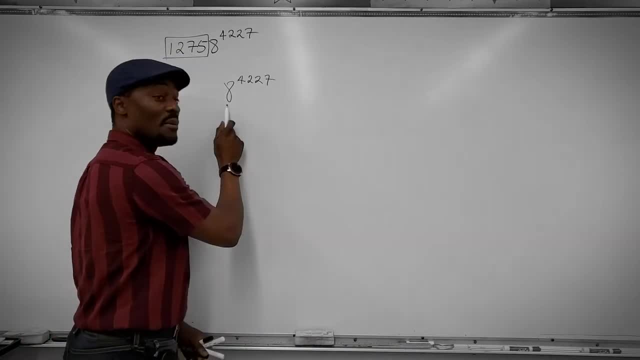 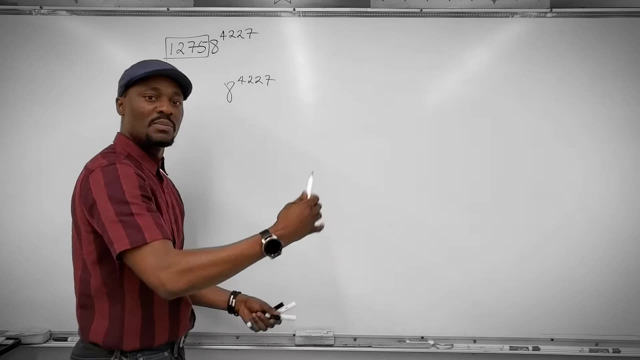 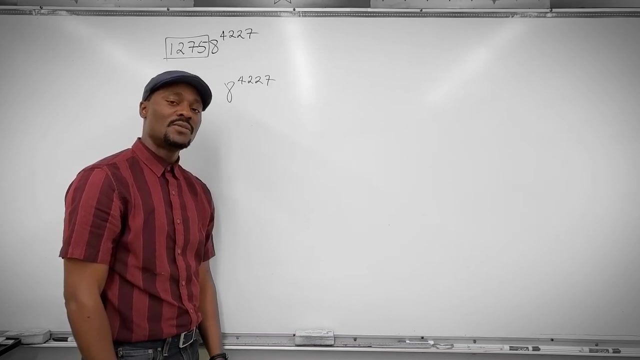 to the problem. the last digit of this number, this number here is basically the same last digit you would get if this was the number you were just multiplying. you were just multiplying eight by itself, four thousand two hundred and twenty seven times. you should feel good about yourself. you just discovered a. 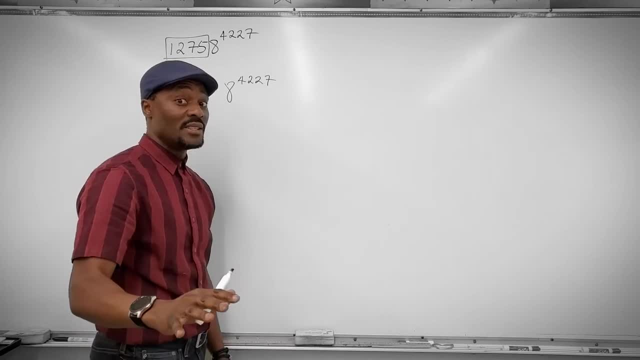 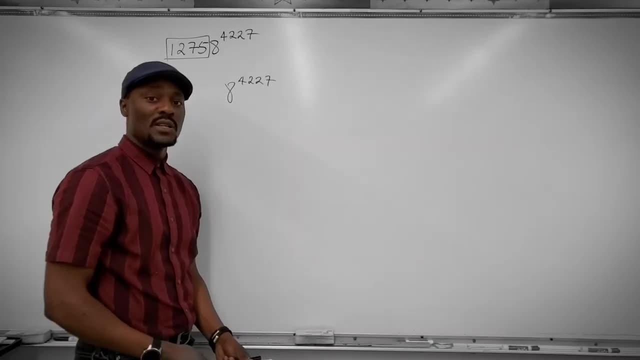 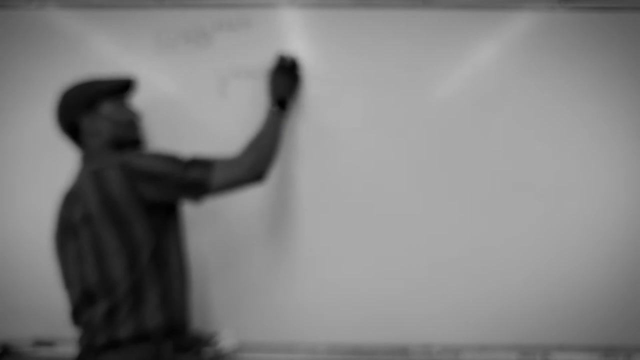 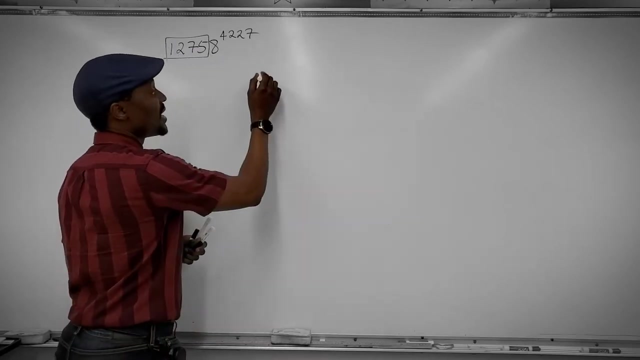 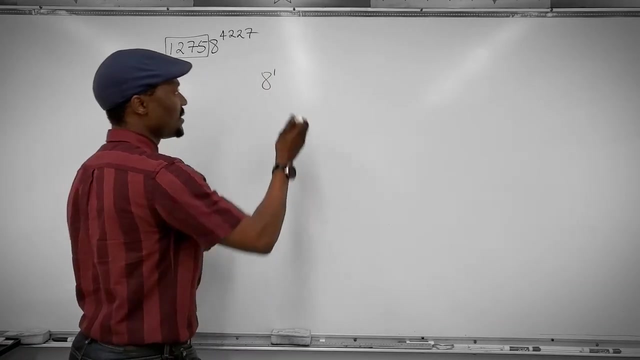 secret. the last digit is always what you need. what do we do if we're supposed to raise eight to the power of four thousand two hundred and twenty seven? let me tell you what you're going to do. and then we go to eight, to the first power. what do you get? your answer is going to be eight. 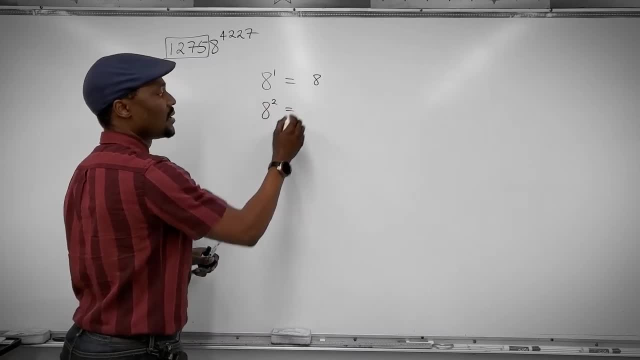 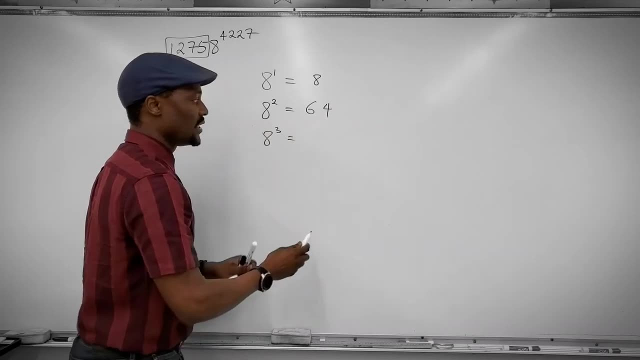 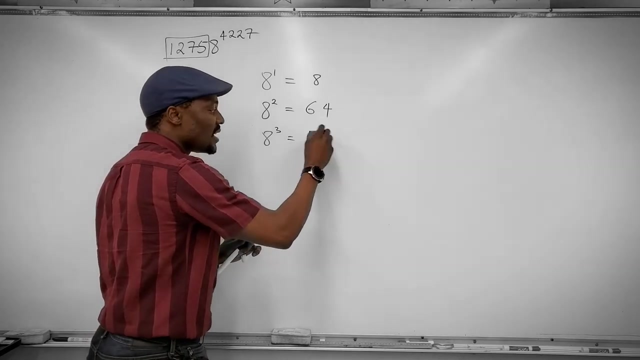 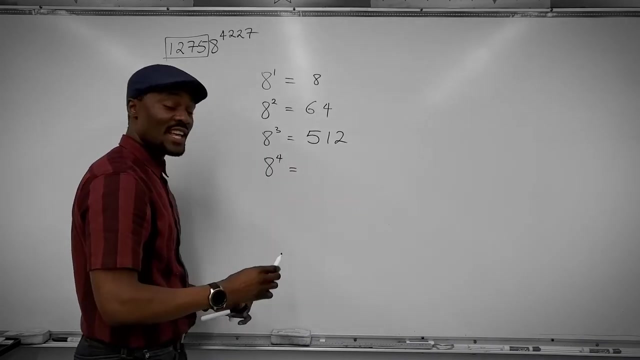 and then eight to the second power. your answer is going to be sixty four and then eight to the third power. if this is going to be sixty four times eight, it's going to be five hundred and twelve. and then you do eight multiplied by four. again, it's going to be five hundred and twelve multiplied by eight. I know the. 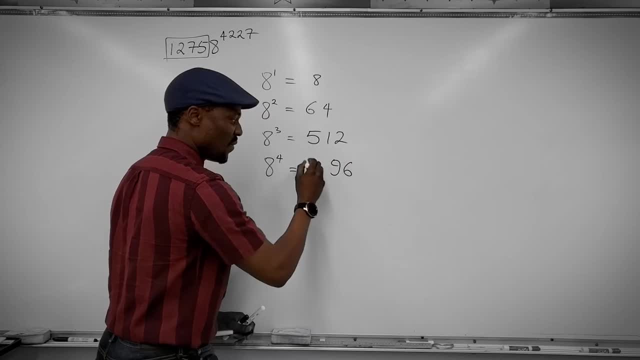 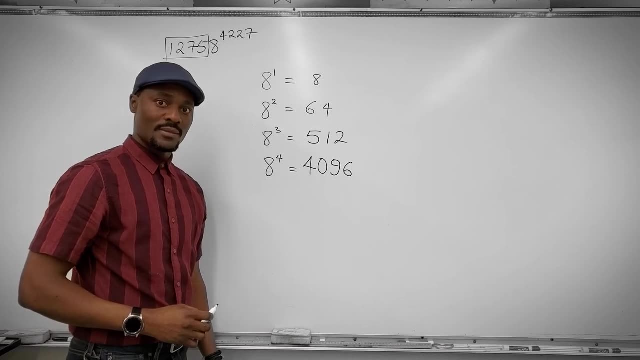 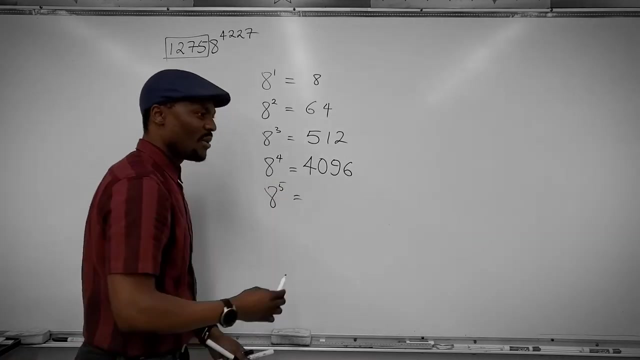 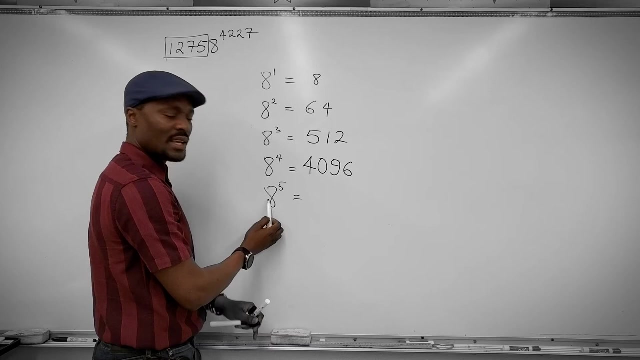 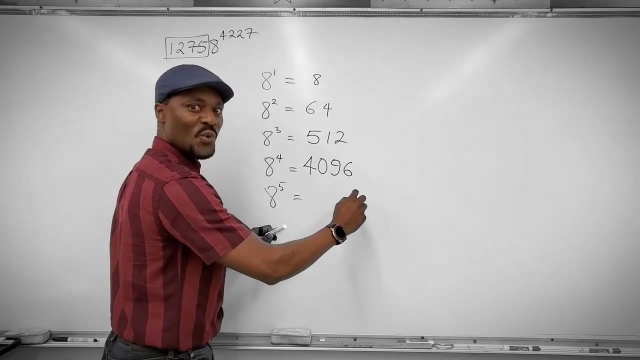 last digit is gonna be six, and it's gonna be four thousand and ninety six. okay, am I stuck? you got to help me. eight to the fifth power. well, I really don't know what. the last? okay, the last digit should be this number multiplied by eight. if I multiply six by eight, I'm gonna get the last digit again. it's. 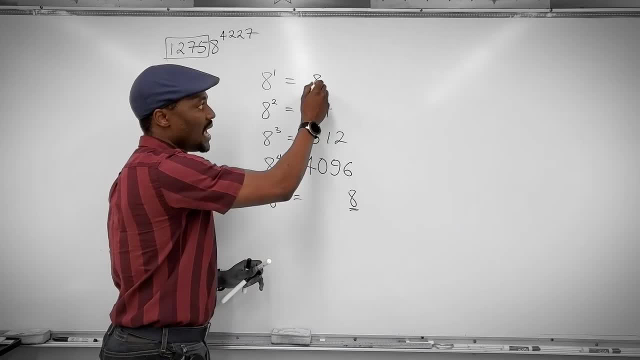 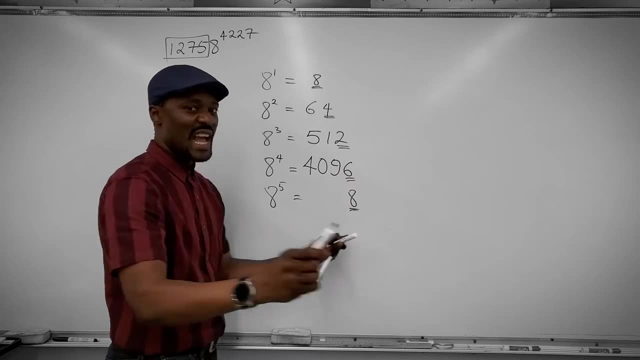 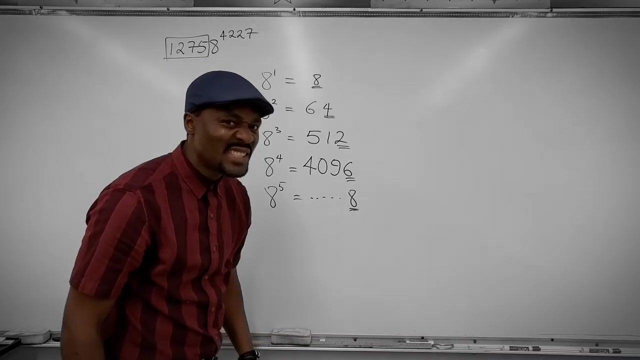 gonna be eight. I started with eight. it went from eight to four to two to six and back to eight, and I can predict that whatever number was here, I don't care about these numbers. what I care about is the last digit. say last digit, okay, so if I go to, 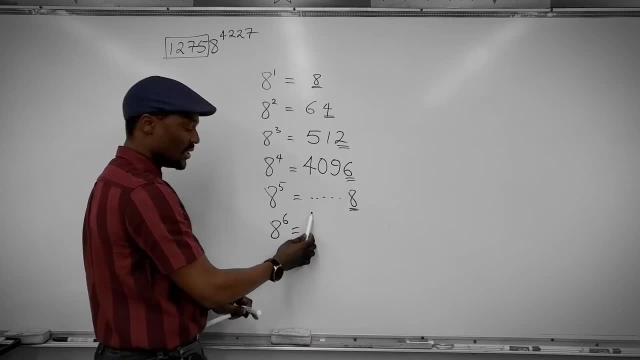 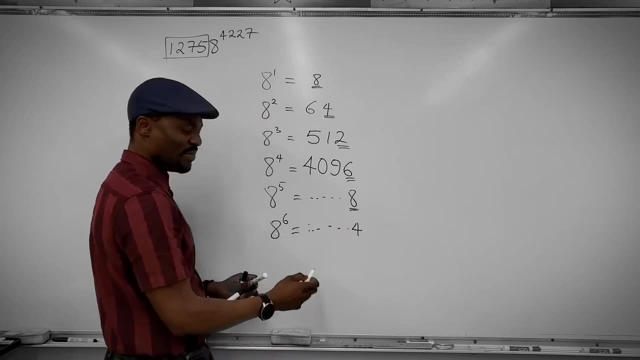 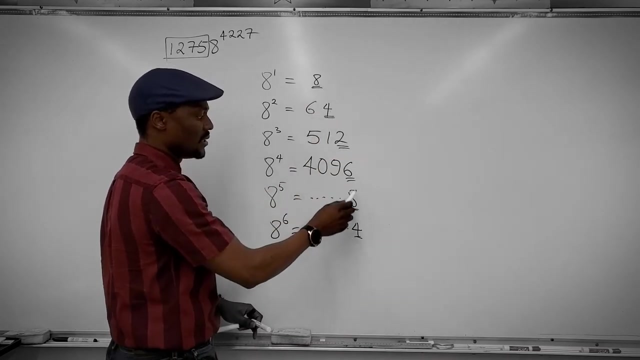 eight to the sixth power it's going to be whatever. this number is multiplied by eight, eight times a sixty four, I'm gonna write four, and then there's another five. i don't want those numbers, i'm stuck with four. so i've gone from eight to four to two, to six to eight. 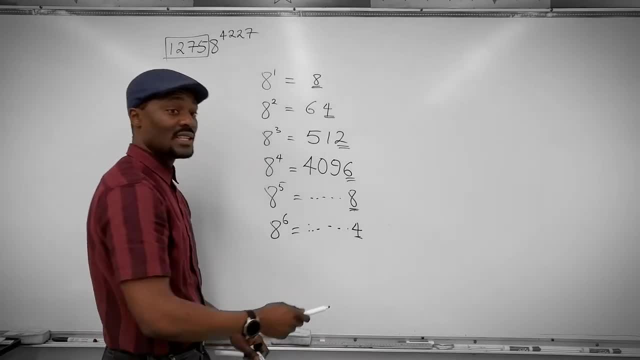 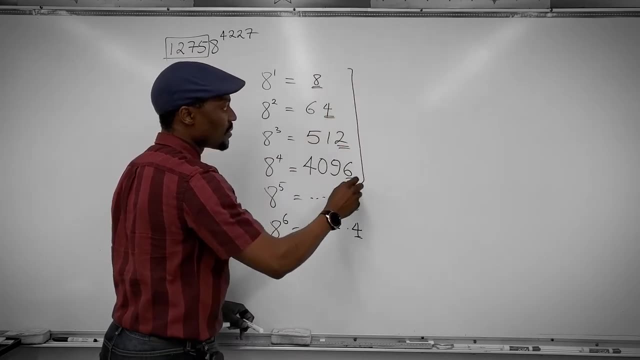 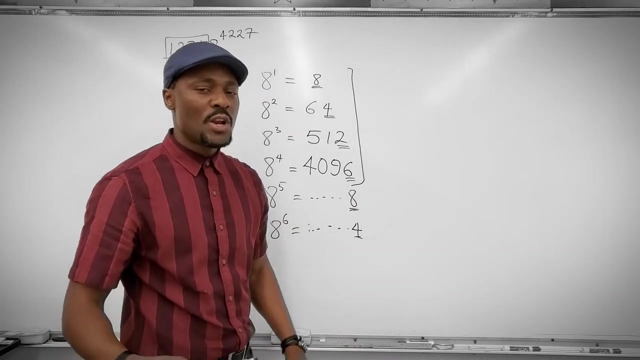 to four, i can predict that the next number will be two and the next last digit will be six. you keep repeating a cycle of four digits: eight, four, two, six, eight, four, two, six, eight, four, two, six. we don't want to keep doing that. we're going to be wasting time and markers and board space. 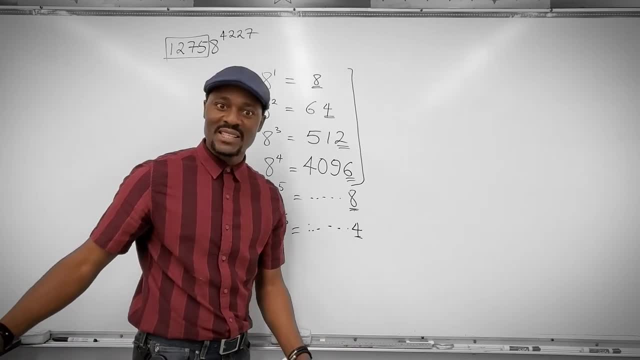 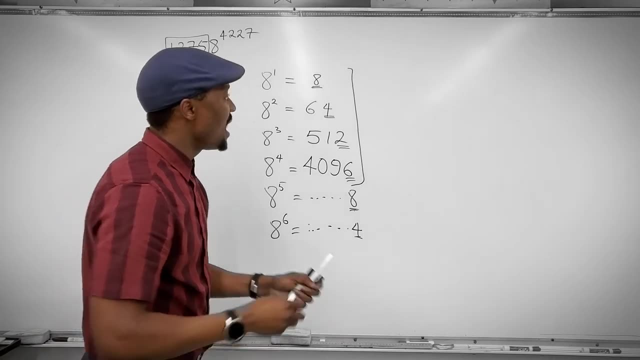 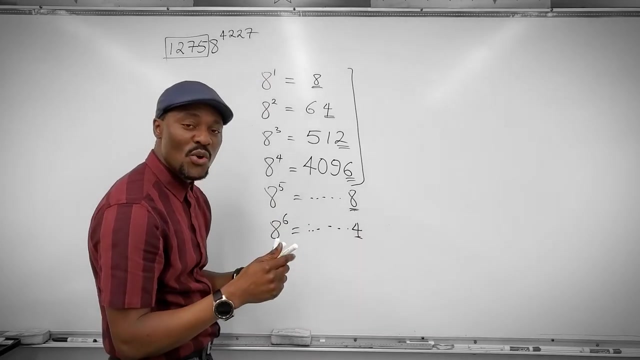 just move on, just move hard, come on. just let the past be gone. okay, so everything else is in the past. all we're dealing with right now is that when you multiply a by itself, many times, all you're just doing is the last digits are repeating. it's either, it's an. 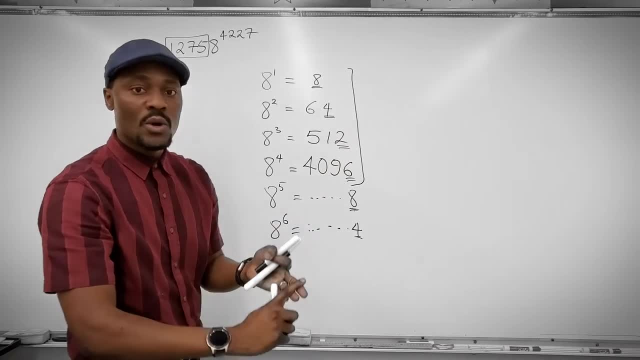 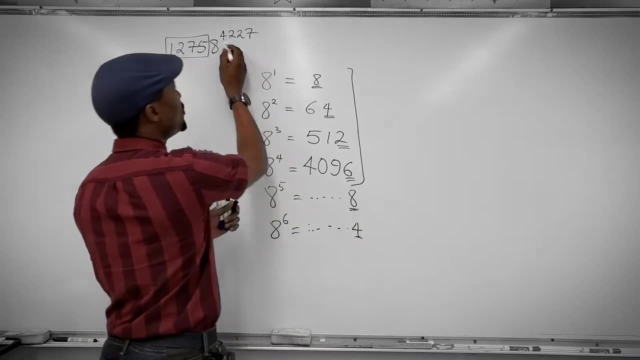 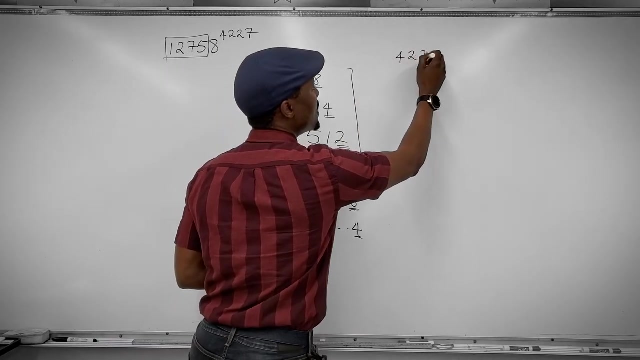 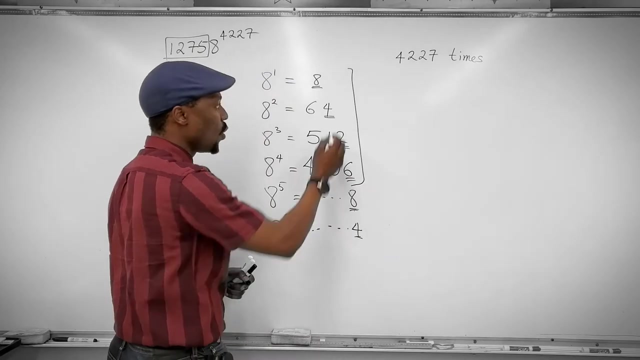 or it's a four, or it's a two, or it's a six, then you start again, then you start again, then you start again. so if you have to do that, four thousand two hundred and twenty seven times four thousand two hundred and twenty seven times, Wow, you just have to go over four and then four. so the first time you're. 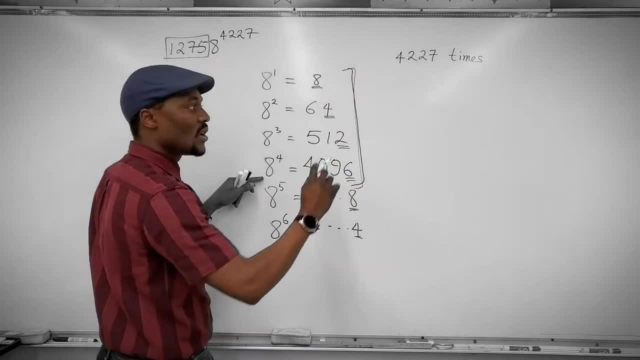 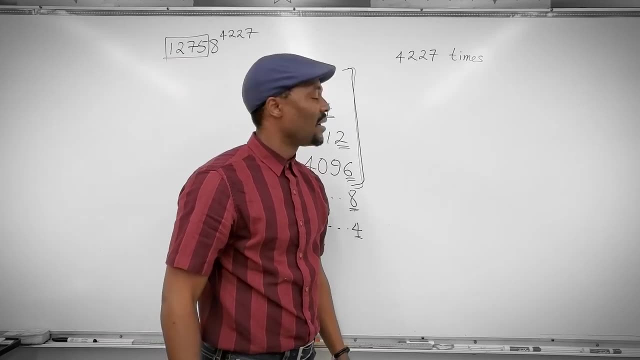 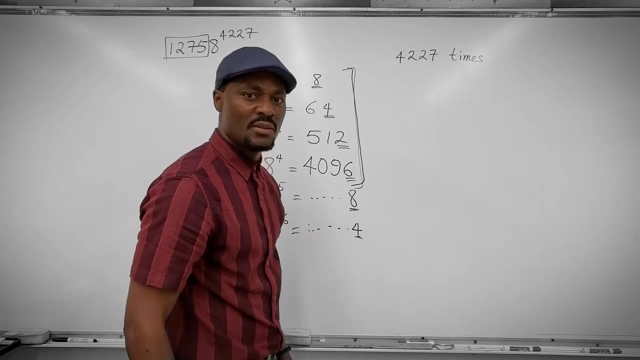 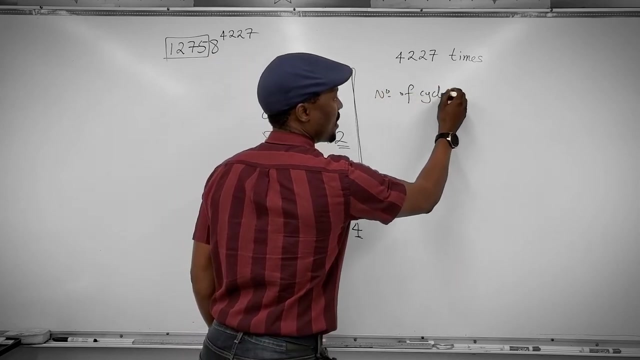 gonna have a cycle of four, starting from eight. then you start another cycle of four, and another cycle of four and another cycle of four. how many cycles of four are you gonna get if you're going four thousand two hundred and twenty seven times? well, you just divide it by four, okay, so number of cycles, number of 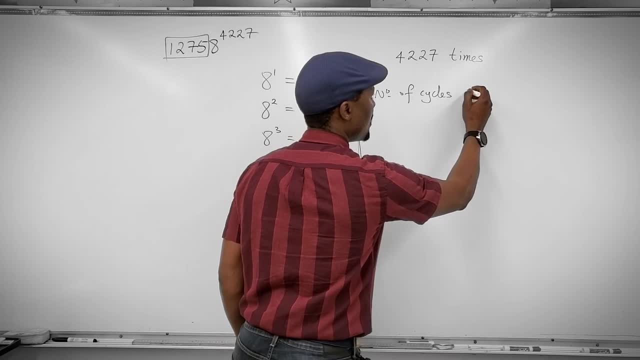 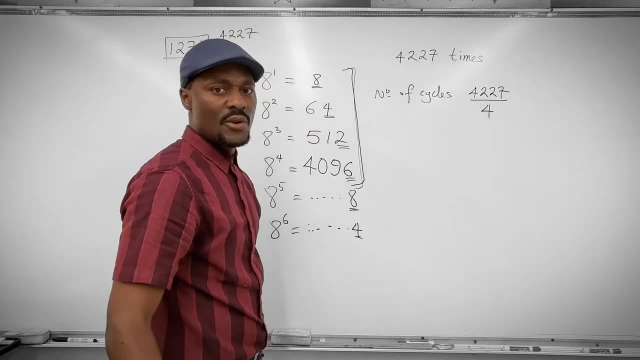 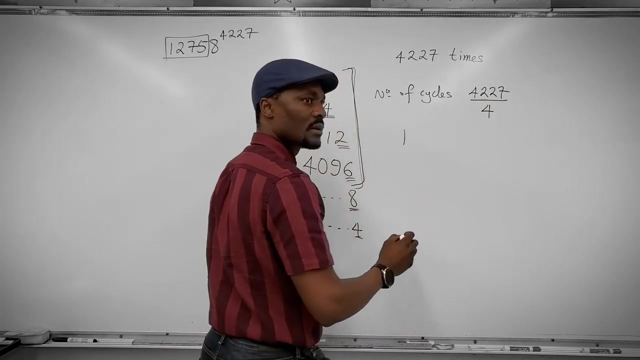 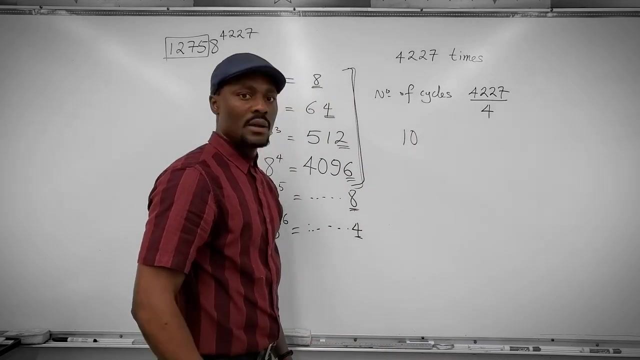 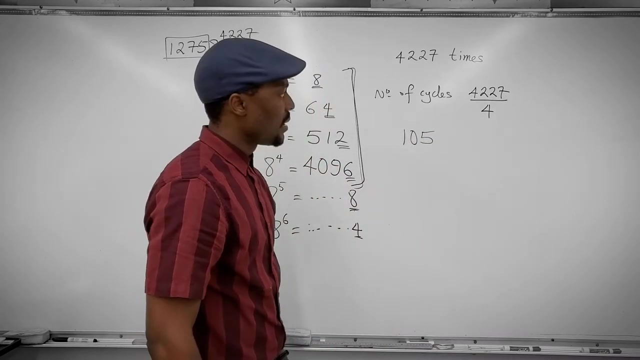 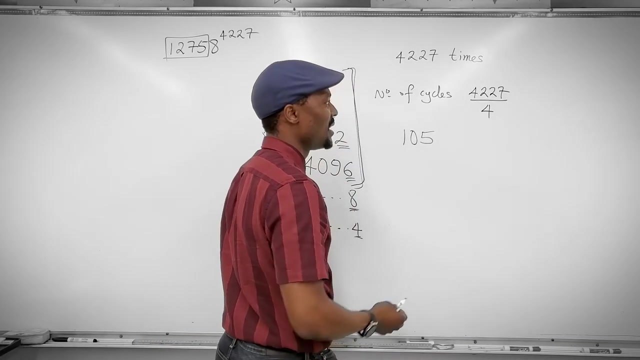 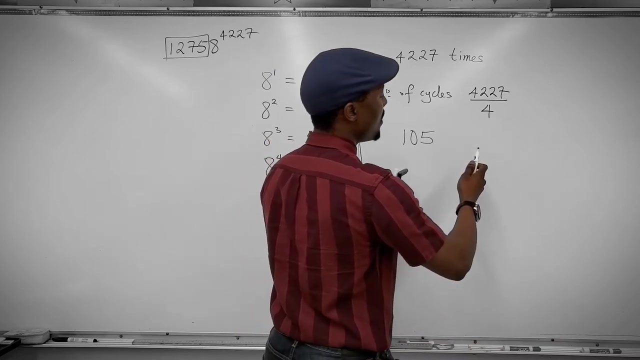 cycles is going to be four thousand two hundred and twenty seven divided by four. now you can help me, thank you. what we got is you divide this by four, you're gonna get one. stop, somebody, help me. okay, it's one zero, it's gonna be five and four in twenty. 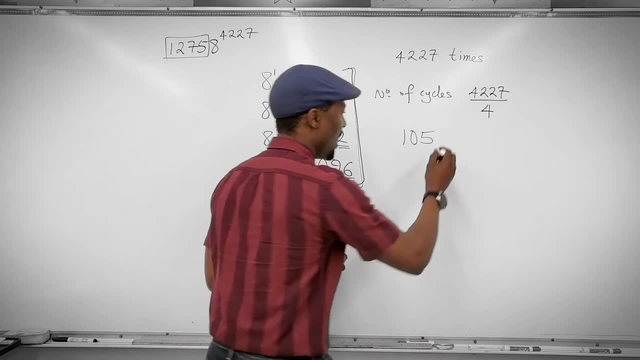 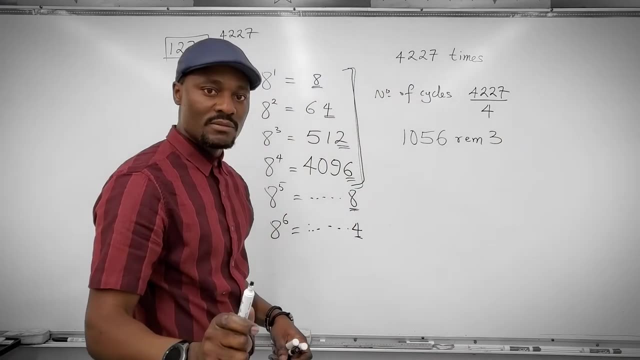 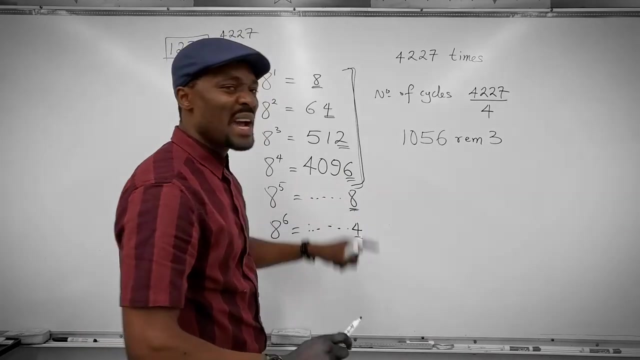 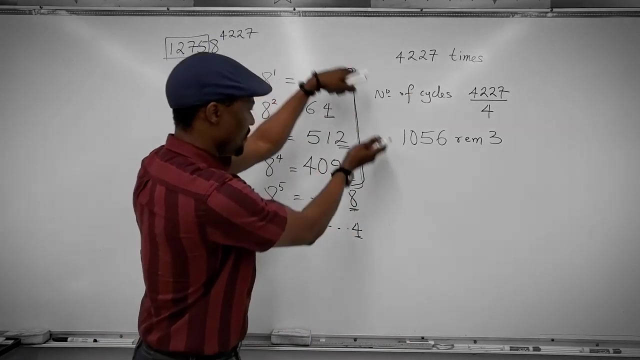 seven should be six. ah, I got that. and the remainder is three. so it means when you keep multiplying, when you keep multiplying eight by itself, you did four thousand two hundred and twenty seven times. you're gonna keep getting cycles of four, you to go over it doing this 1056 times and there'll be a. 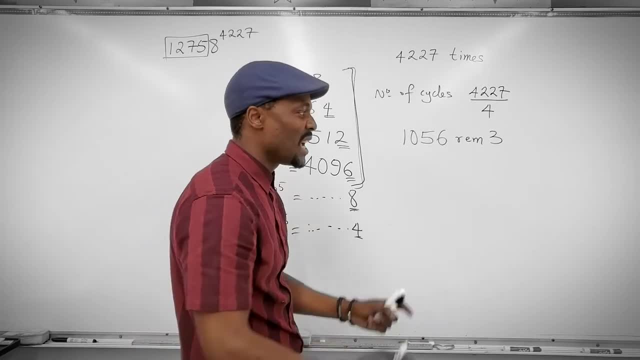 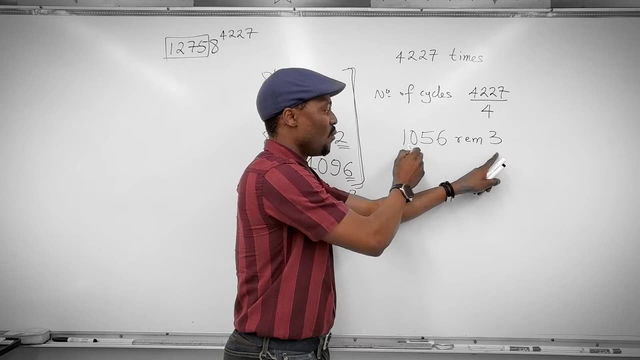 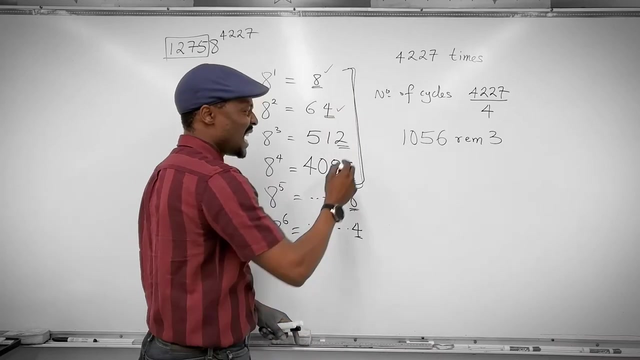 time where it will not complete the cycle, because you can't multiply four times, you can only do it three times. so the first time after this 1056 time, the first time- is going to be eight. the second time, your last digits will be four and the last, 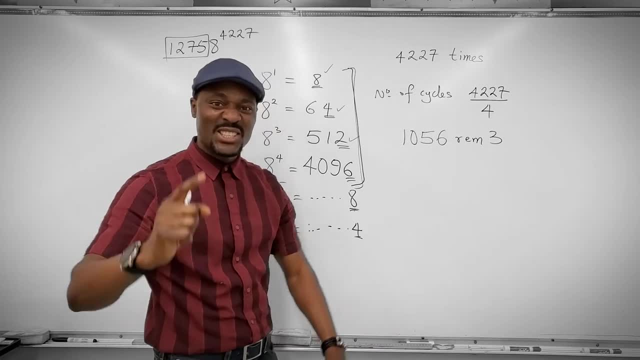 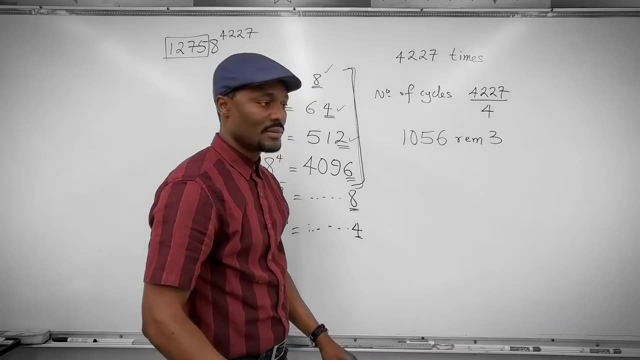 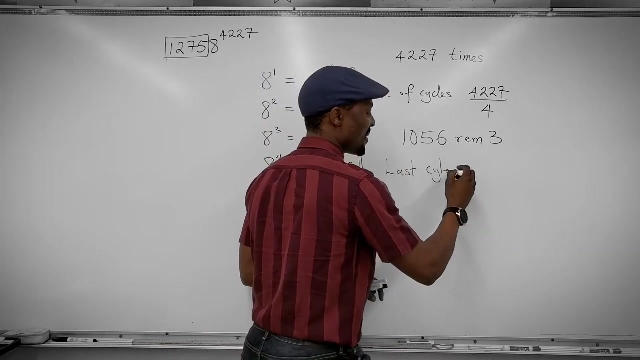 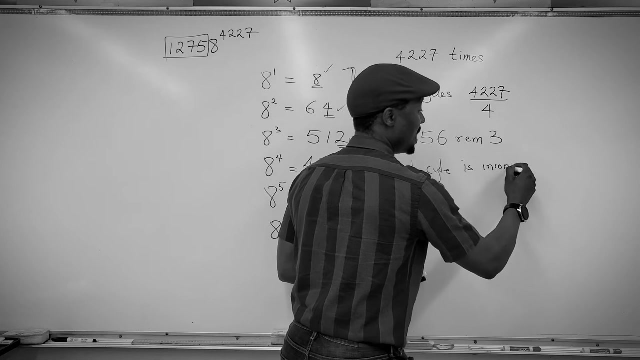 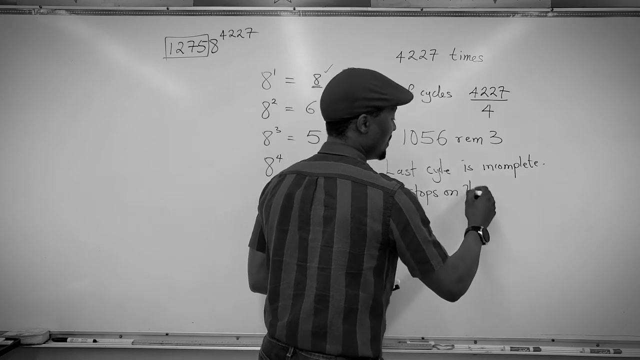 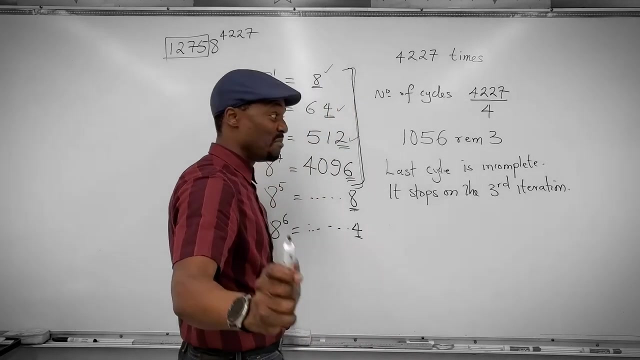 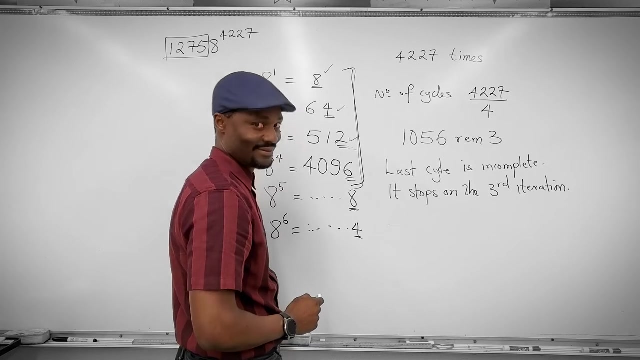 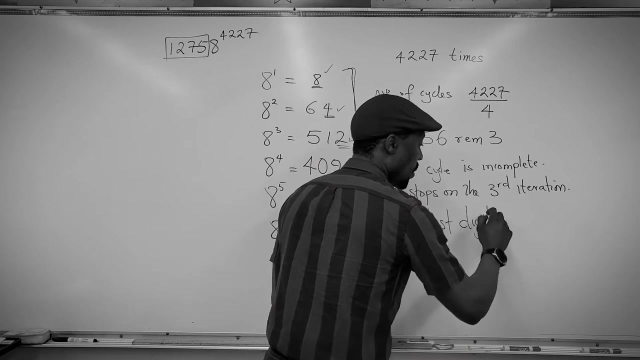 time, which is the third time, the last digit is gonna be three, not three, it's gonna be two. don't put your answer wrong: cycle last cycle is incomplete or it stops on the third iteration. okay, if it stops on the third iteration, it means that you actually got this third number, the last digit, who is two if you? 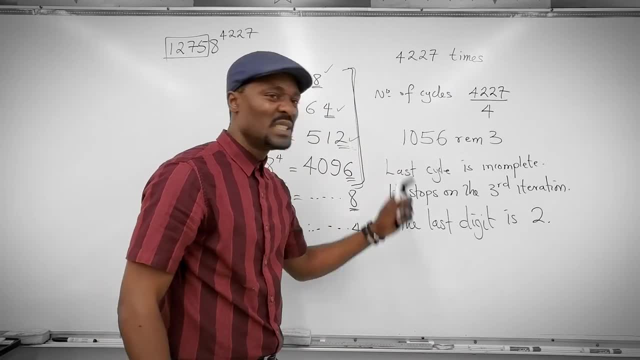 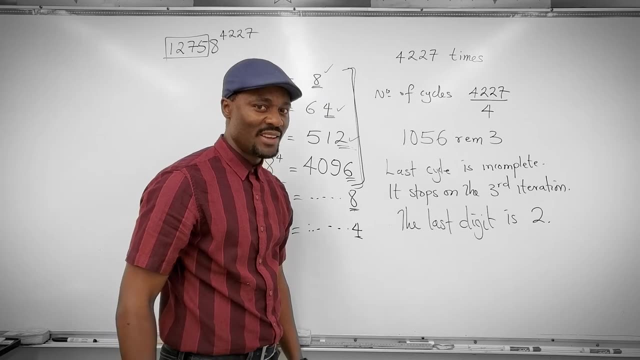 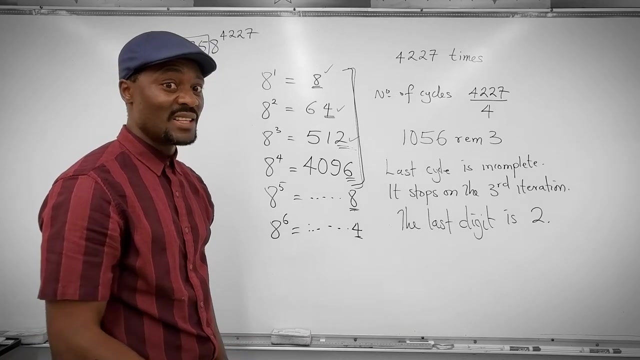 have a supercomputer. we have a computer that can give you a, the digits. punch it in, let's see what you got. punch it, let's see what you got. okay, that's a very straightforward example. let's take another example. if you didn't get this, i'm going to 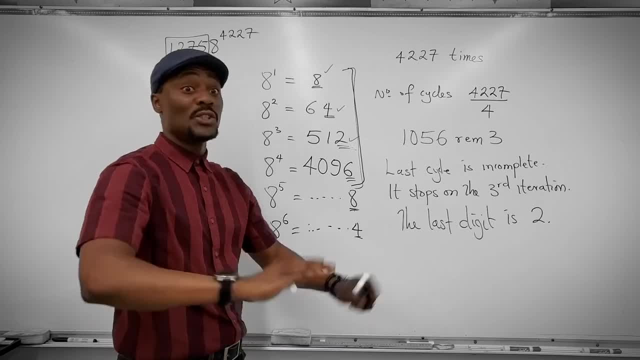 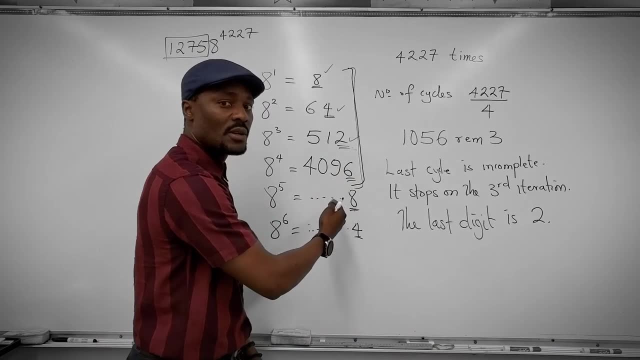 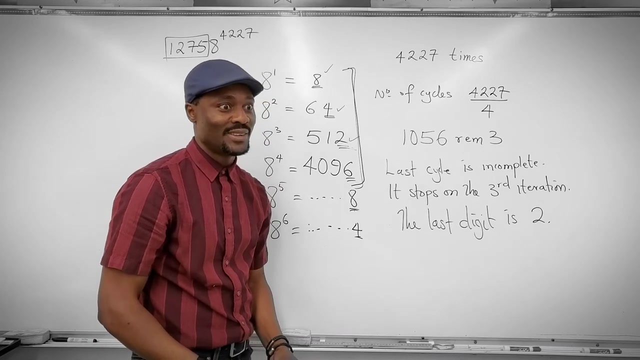 use a simpler example for you to get it, and then i'll show you the trick to all questions. okay, any question, any number, you can find it. you just first need to get the cycle. when you get the cycle, it makes you cool. the cycle makes you cool, that's cool. okay, let's go on. okay, so i'm gonna. 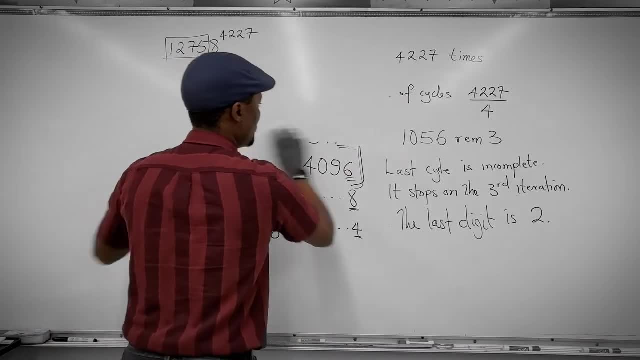 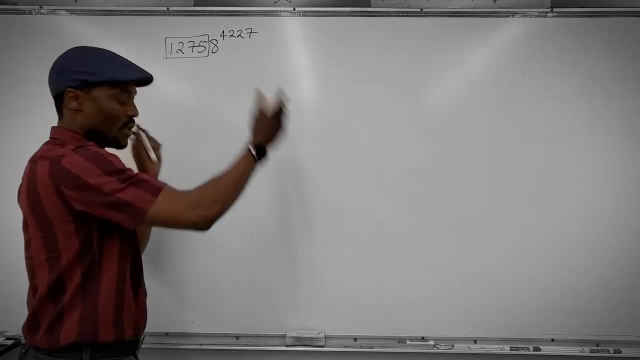 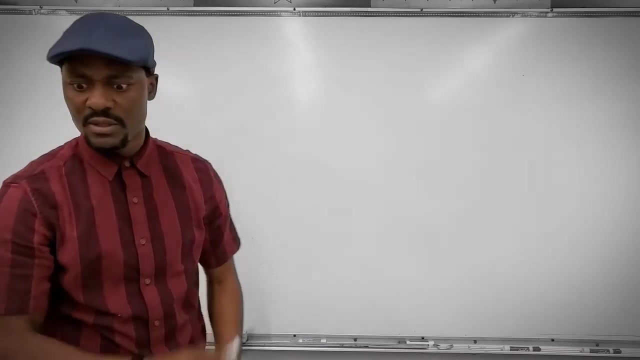 i've just erased this because i believe you got this and then i'll show you something else. okay, so we just answered this question. we don't need you anymore. the problem we created, we solved you. you can't, you can't, don't mess with this, let's go on. 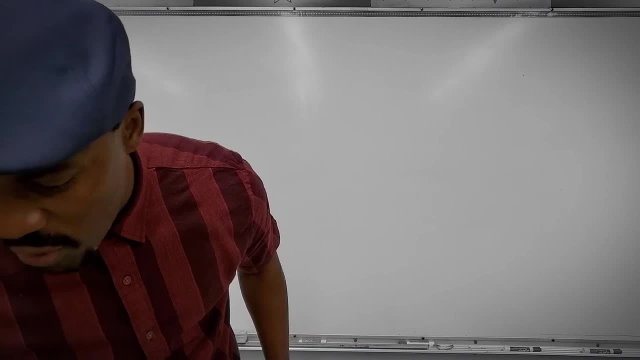 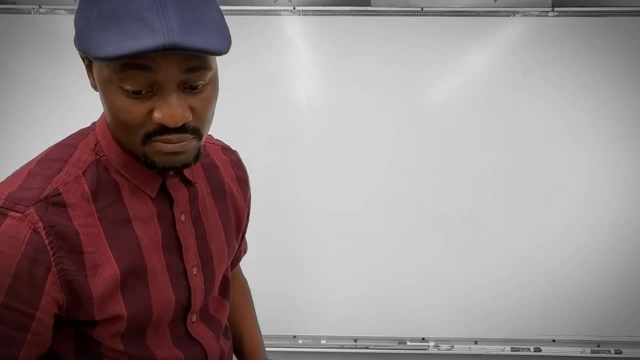 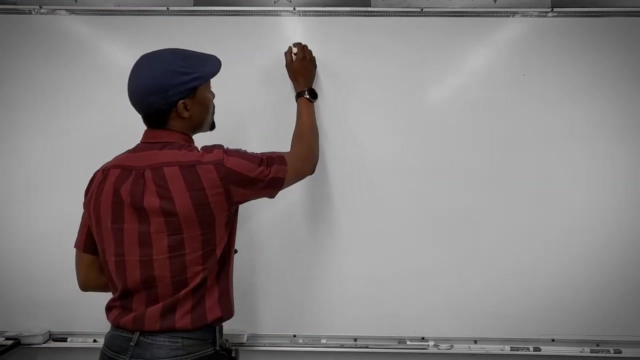 let me look for another example that i was trying to work on and i thought, okay, maybe this would be much easier for people to understand. i can't find the problem i created. see, always track your problem. so i'm just going to give you, um, a number like two, three, nine, six, okay, so let's try: two, three. 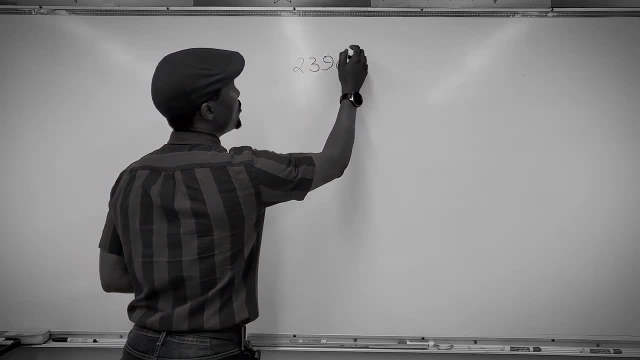 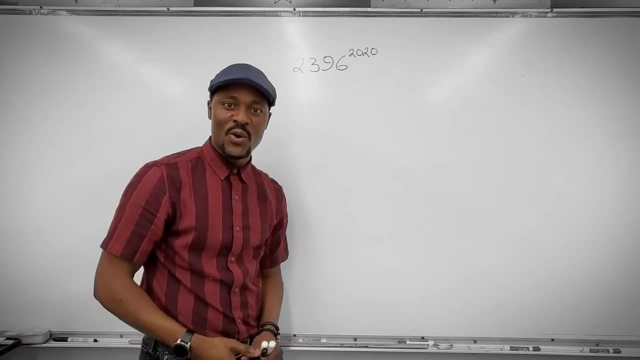 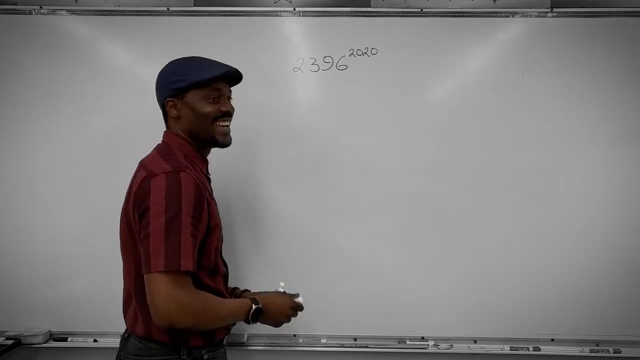 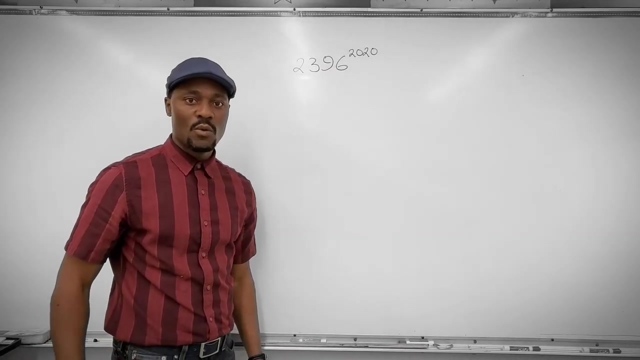 nine six race to power 20- 20.. that's next year. if you're watching this video in 2020, you know that i created this problem in 2019 for you. okay, so this is it. remember. all the digits before the last digit are not relevant to the problem. what is the last digit when you raise 2396 to the power 2020? 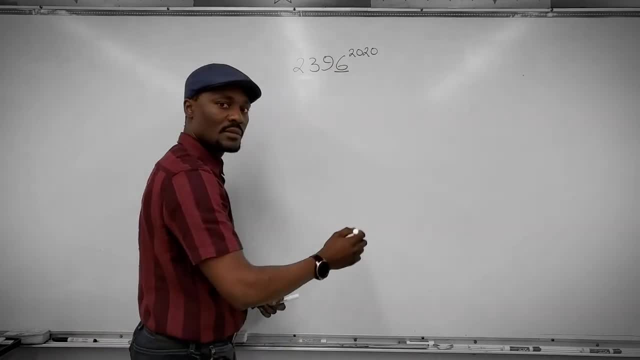 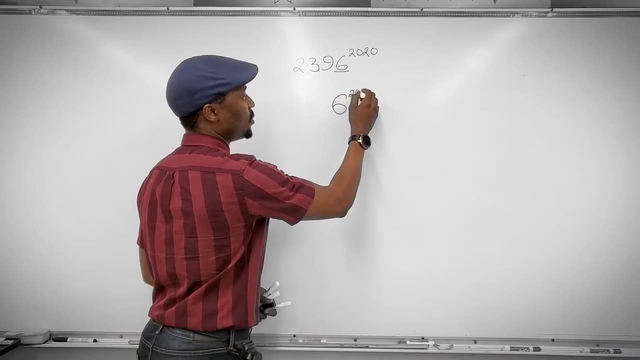 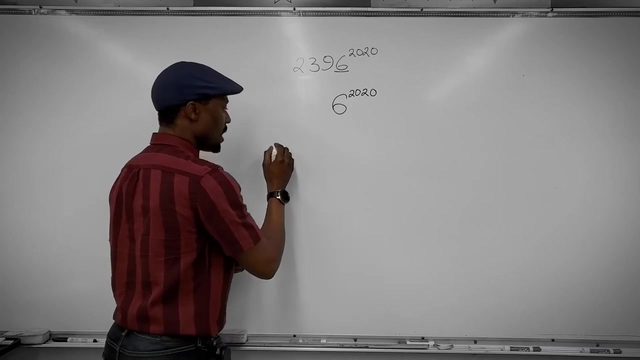 well, my business is with mr six. so i'm just going to say the last digit will be determined by six to the power 20, 20.. then i need to find the cycle for six. so i go: what is six to the first power? it's going to be six. 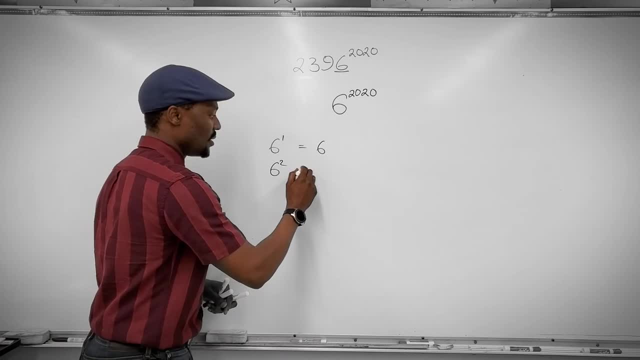 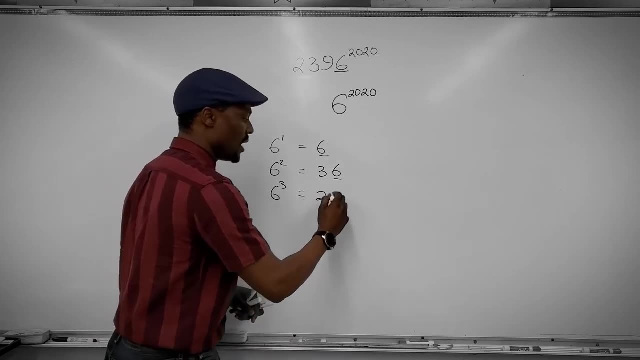 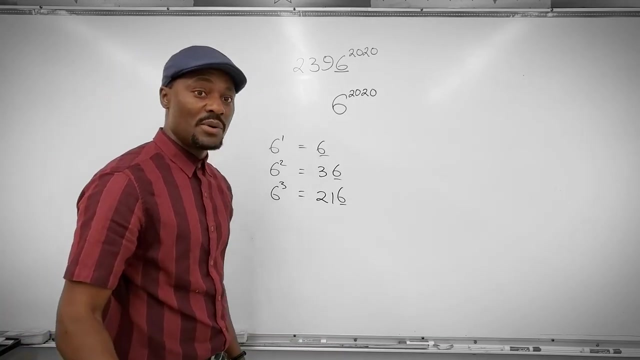 what is six to the second power? it's going to be 36. uh-uh, i got the same digit. what about six to the third power? it's going to be 216 of there is no hope. the last digit of any number that ends in six raised to power, any number will always. 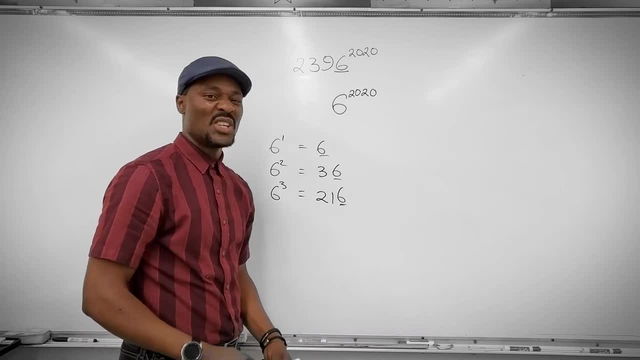 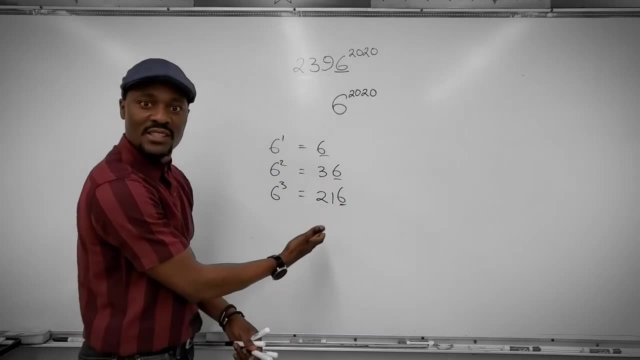 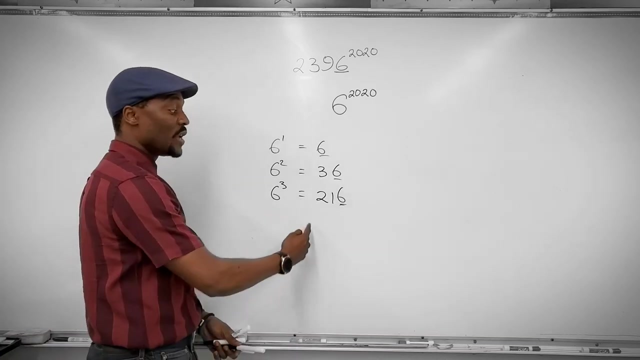 be six. you don't need to do any calculation, you're done with number six. six, uh, just just stay away from us. okay, you're not helping us. so six will always be six. there's another number, two other numbers, three other numbers that will always behave like this if a number ends in zero. 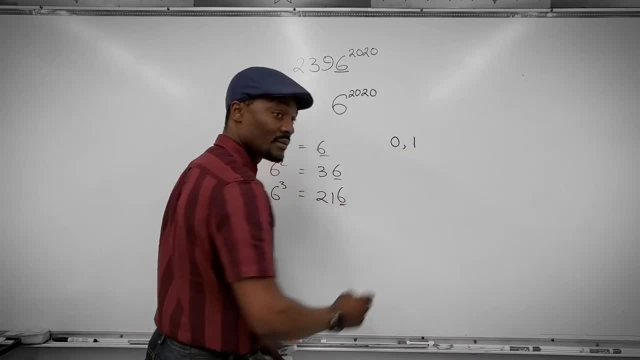 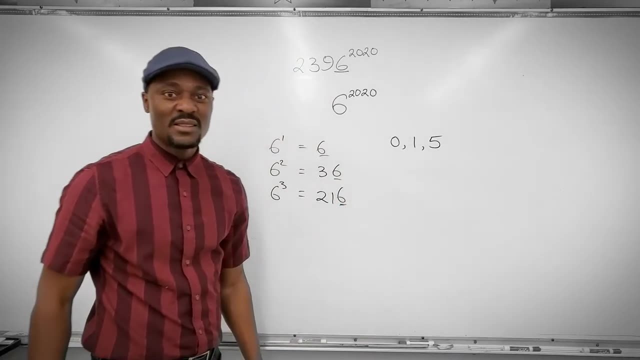 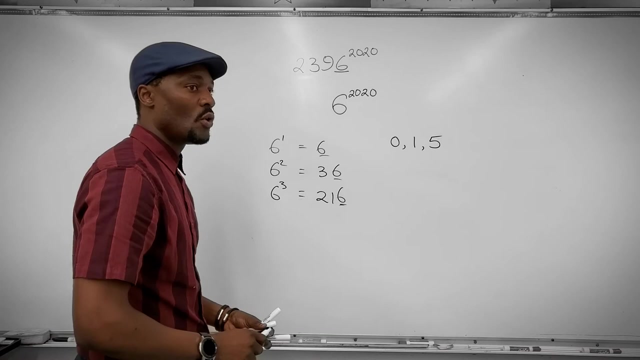 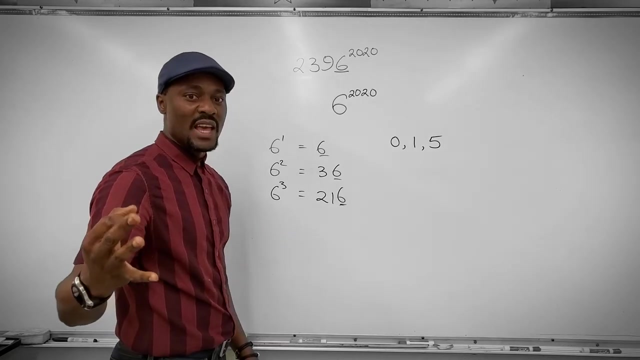 if a number ends in one, if a number ends in five, they will always have the same last digit, no matter what power you raise them to, always have the same last digit. remember that: zero one, five and six. zero one, five and six: always the same last digit. remember that. 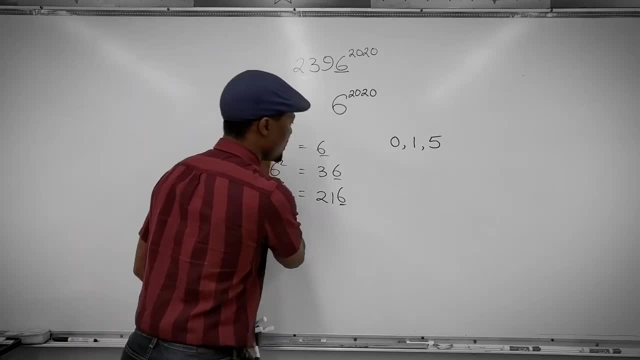 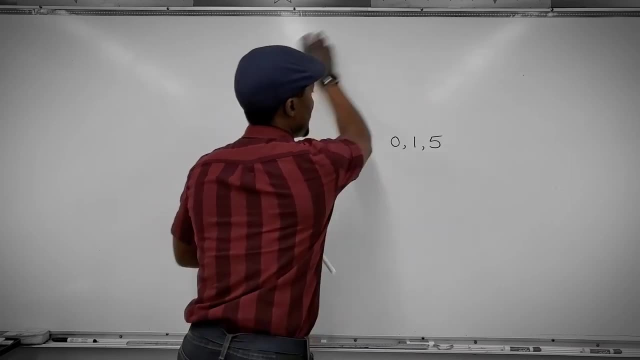 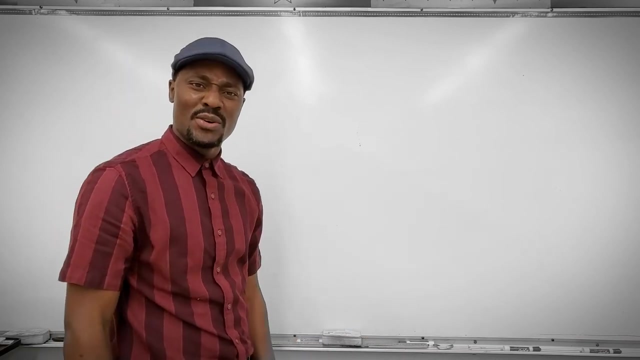 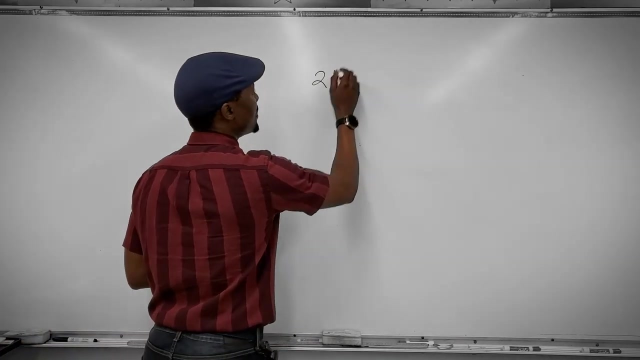 let's move on. come on, I'm gonna get rid of this. let this be in your head, not in your notebook, in your head. so let's go to another problem. let's let's see what happens with mr. let's do some for, okay, what is? 214 raised to power 153. 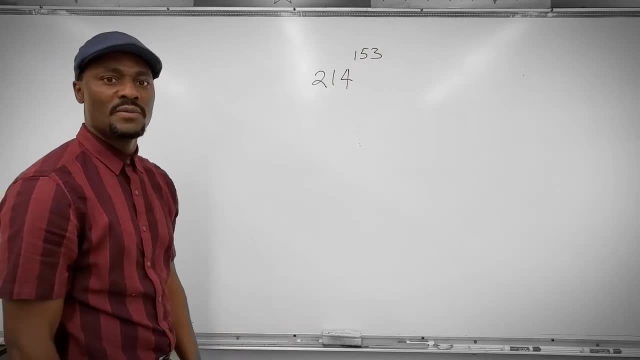 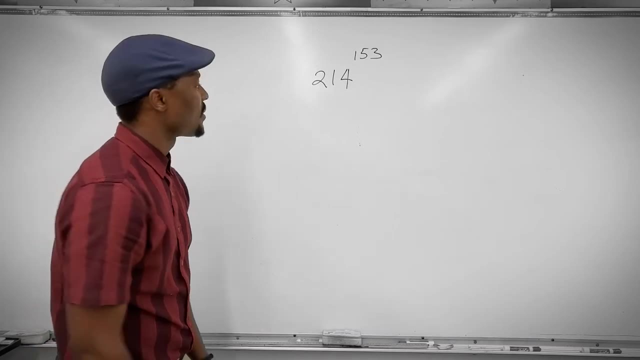 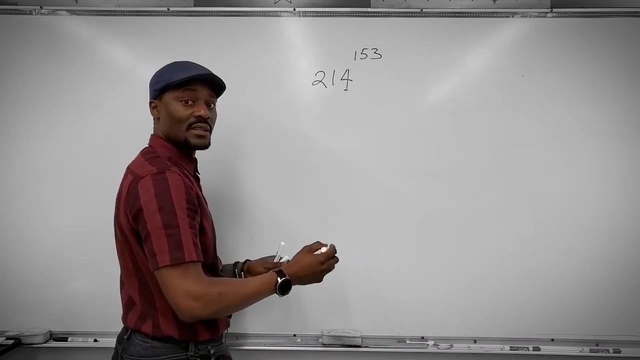 something like that: 214 raised to power 153. let's see, it's gonna be the last digit again. forget about whatever comes before that, stick to the last digit. the last digit is 4. so what is 4 to the first power? 4 to the first power is 4. 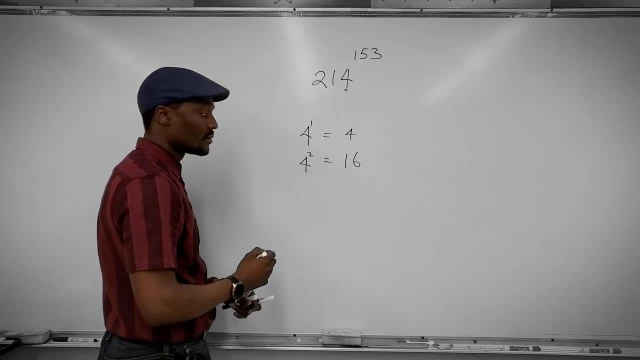 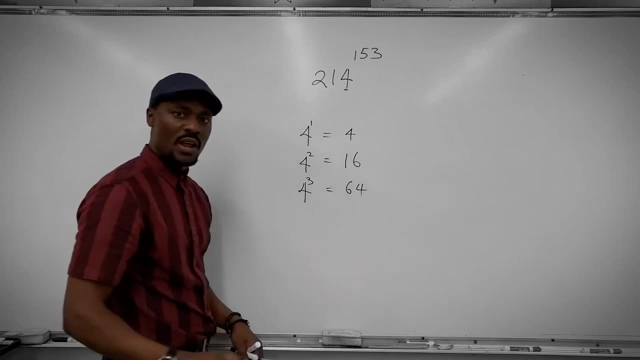 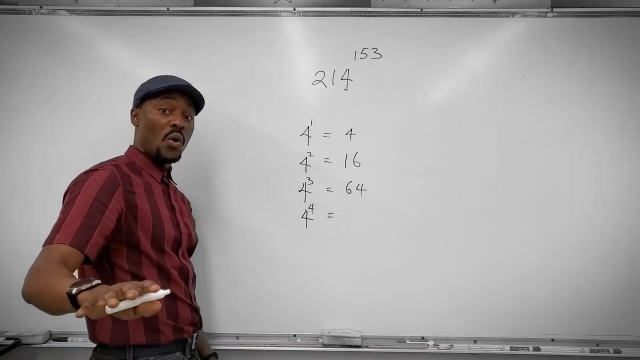 4 to the second power is 16 mmm. what about 4 to the third power? that's 16 times 3 times 4. I know the answer is 64, 4 to the 64 times 4. your answer is gonna be 256. 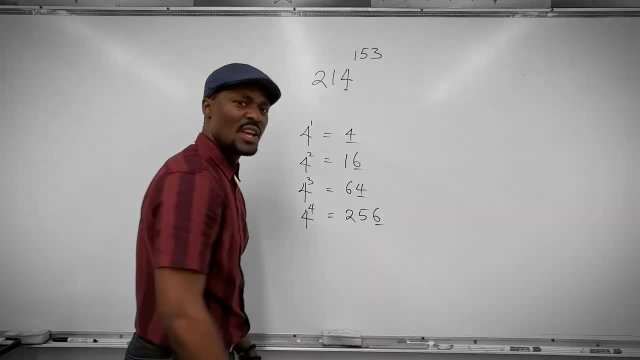 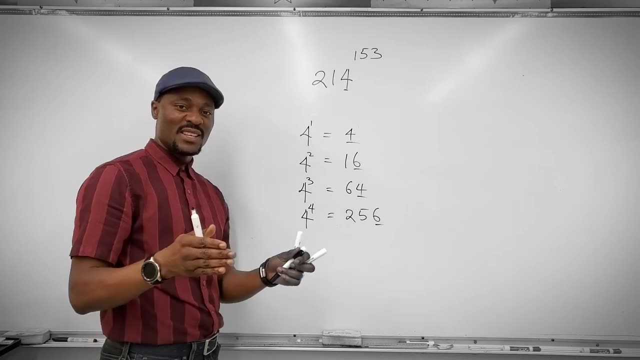 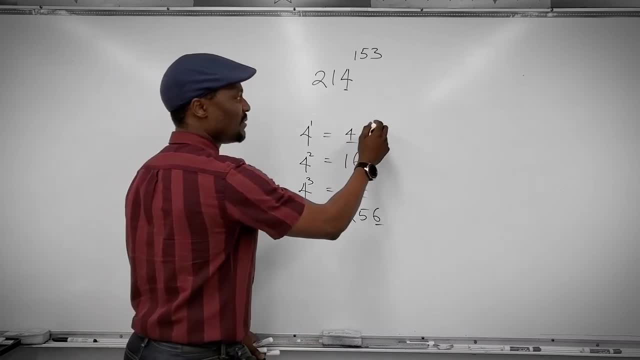 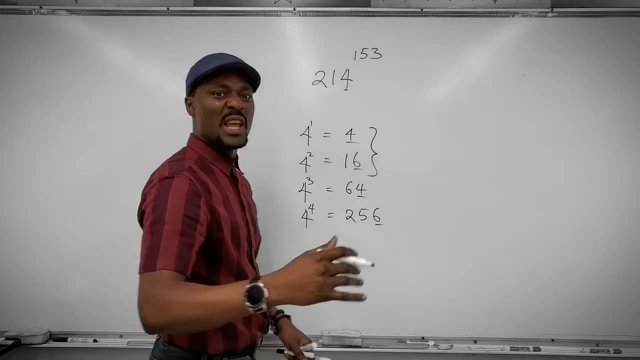 you just gonna keep going. four, 6. come on the cycle length. you have two digits, you just go for 6. okay, how many cycles? how many times are we going to do that? if we're doing it 153 times, we're gonna get this whole for 646 153. 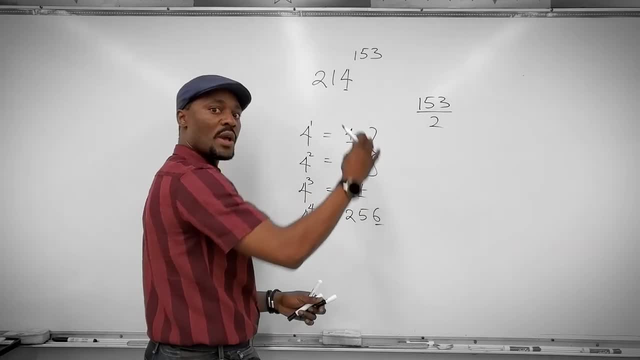 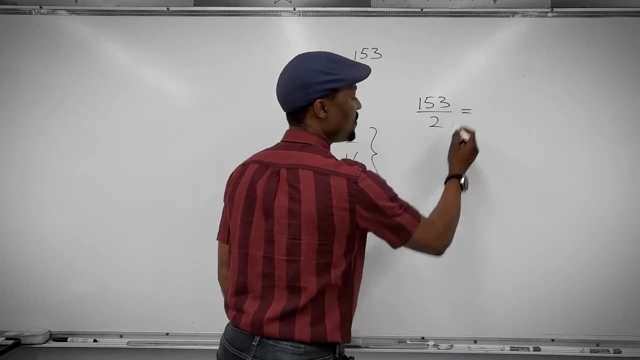 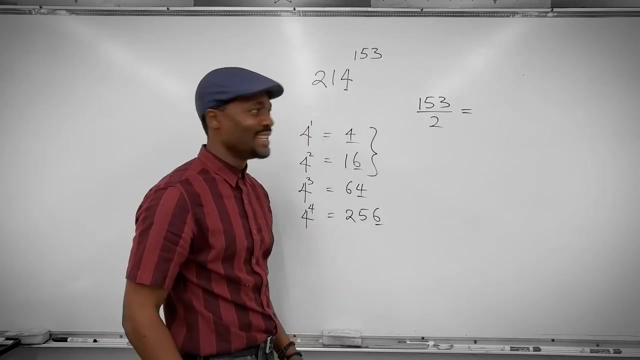 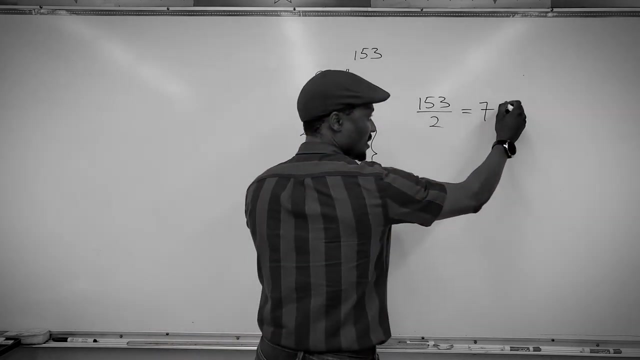 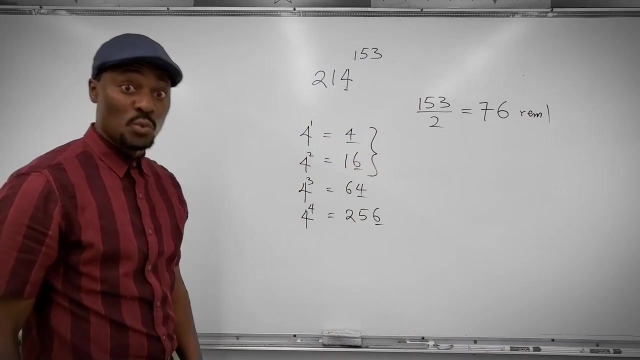 divided by 2, because there are 2 digits that keep going back and forth, back and and four, my friends who fight. 153 divided by two is gonna be. somebody helped me. seven mmm, six, remainder one, this one remaining. if there's a one remaining, it means after you've completed the cycle of four, six, four. 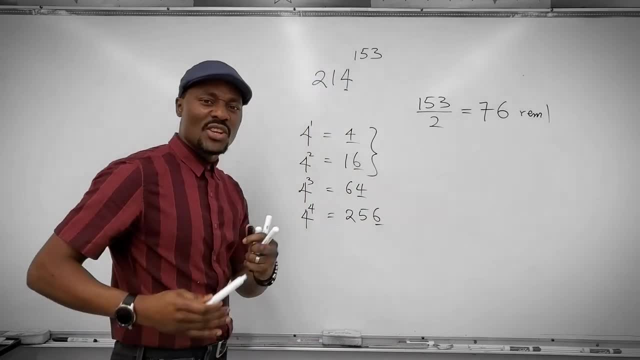 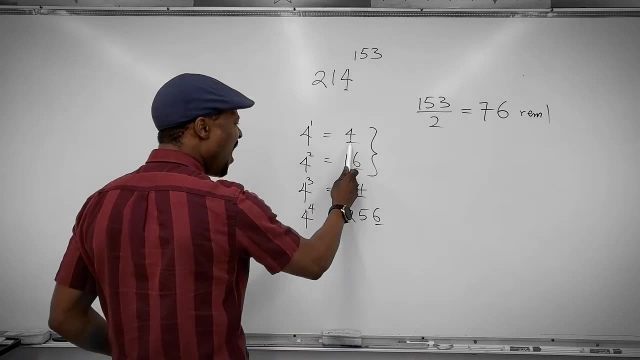 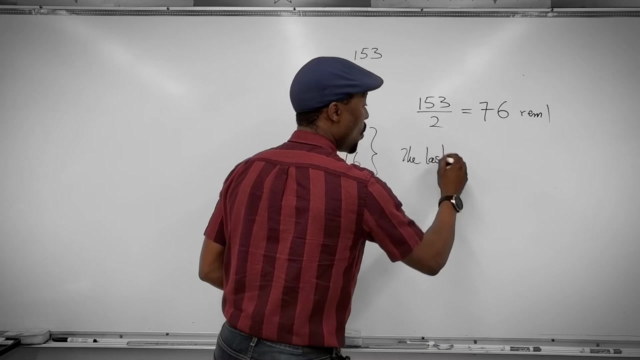 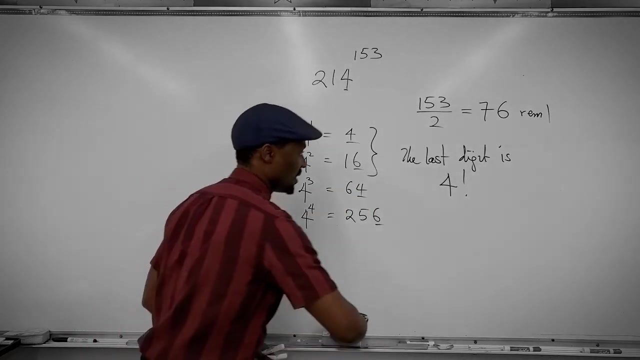 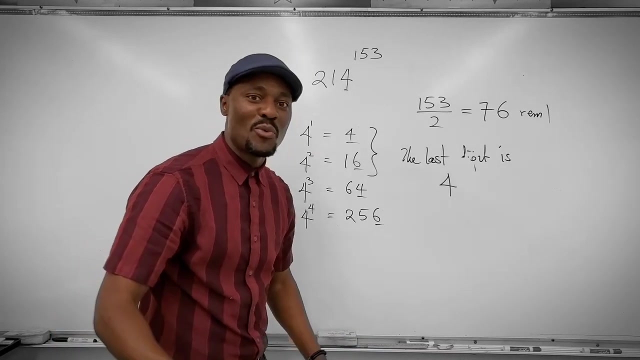 six. you've done that 76 times. the next time you want to stop the cycle? we got the answer. so the last digit, whoo, the last digit. it's gonna be four, not four factorial. that's terrible. come on, don't do that. this is math, not English. I'm excited. how do I write exclamation after I write? 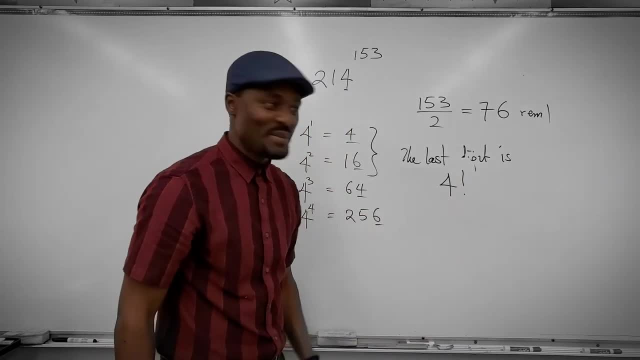 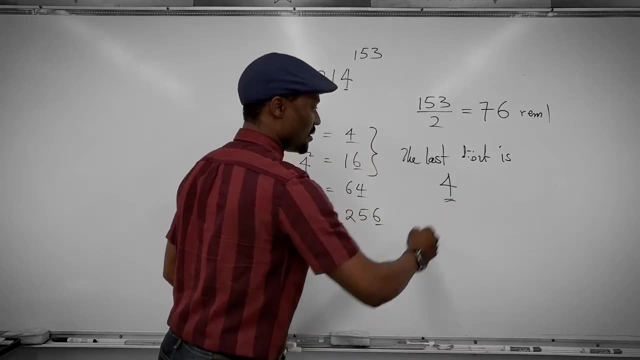 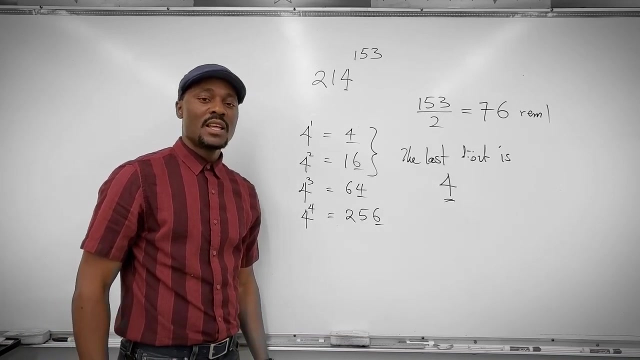 a number in math. I can't do this because that means 24. yeah, okay, don't worry about that. so that's my answer. you want to try another one by yourself? let me just give you the secret of solving all these problems. you just have to know what cycles exist. 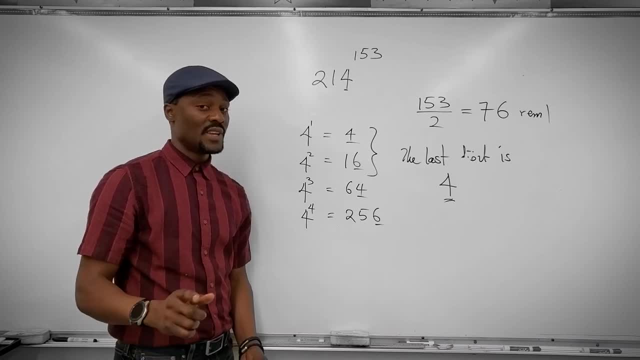 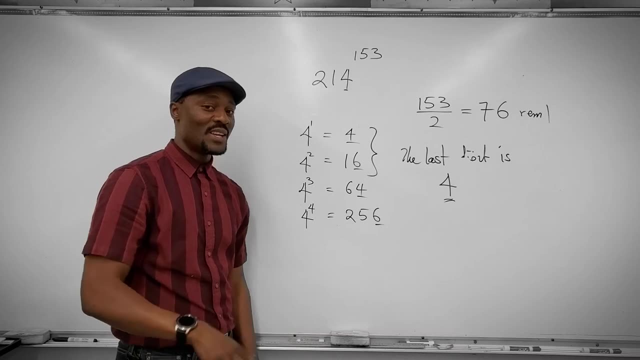 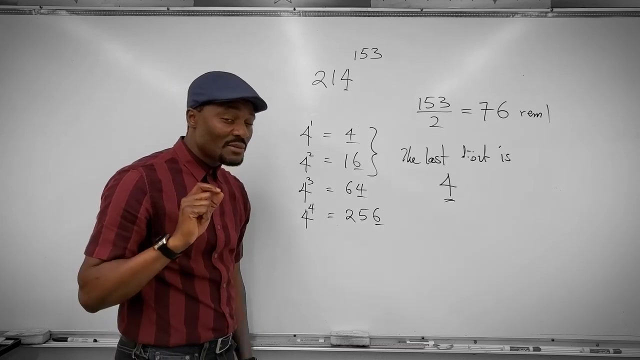 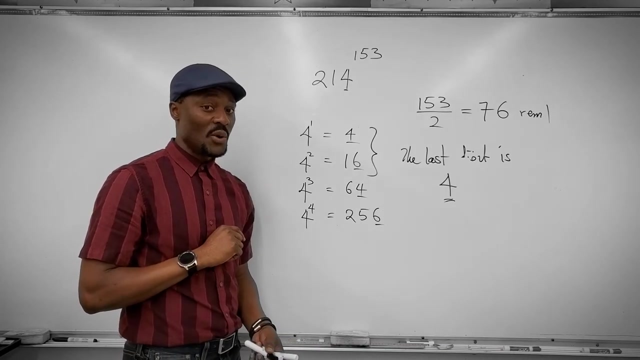 and we will be good. please don't forget to like this video. if you have any comments of how I can improve my videos, please make sure you leave it in the comments. hit the like button. make sure also that you subscribe and you can touch that Bell so that when I upload the next video, you will get a notification. okay. 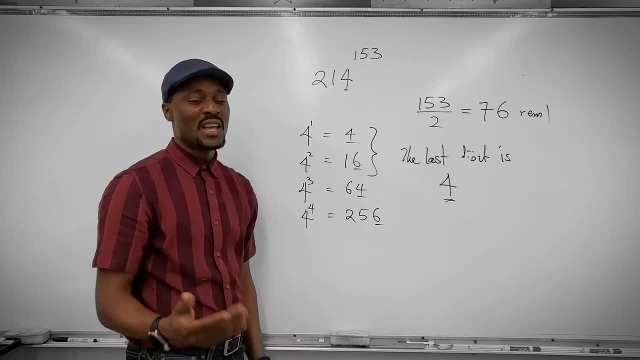 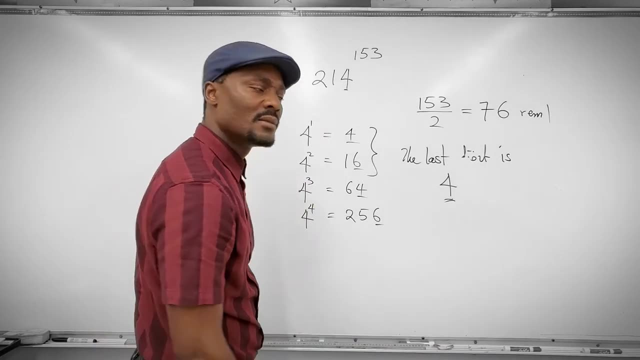 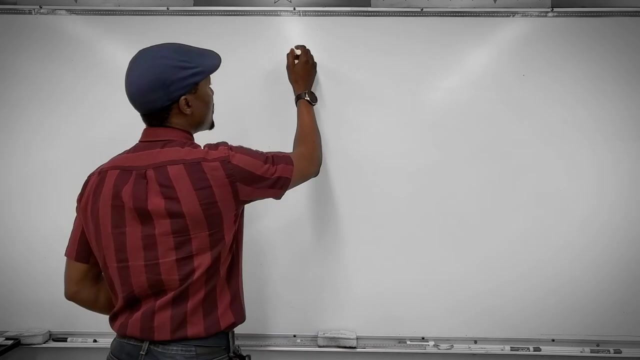 let me give you the secret of all the digits that we use and how they work. so you want to know how to solve a problem. you want to know how to solve a problem. you want to grab your notebook or just put it in your brain. number cycle, the. 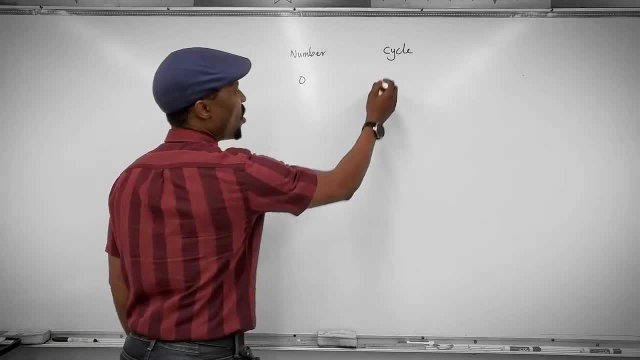 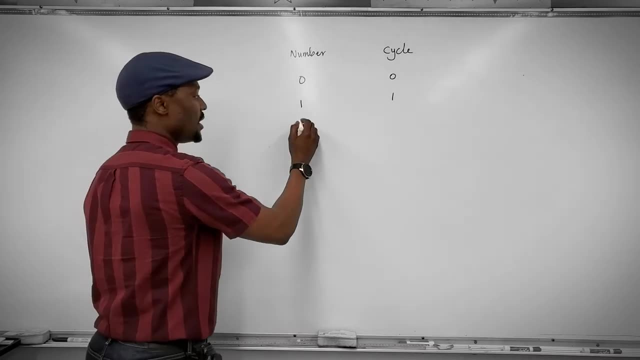 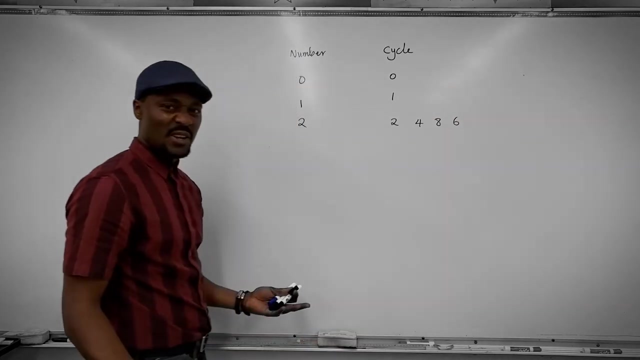 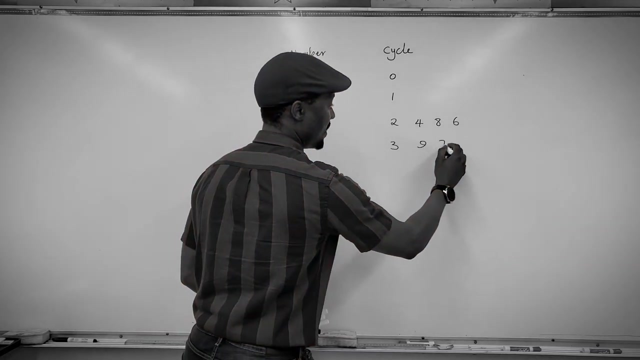 first number is zero. oh well, you'll always have zero. the second number is one: you will always have one. the third number is two. you will always have two, four, eight, six. it's a cycle of four. the third number is three. you will always have three, nine, seven, one. the fourth number is four. you will always have four. 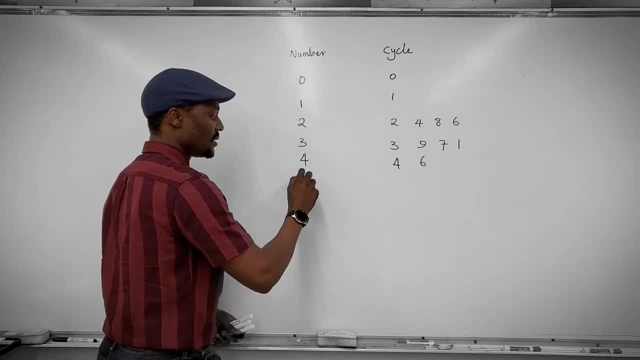 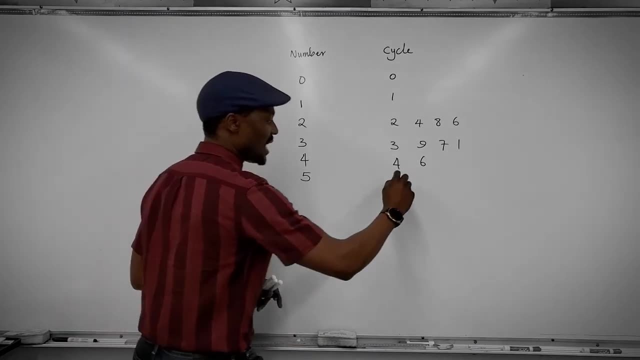 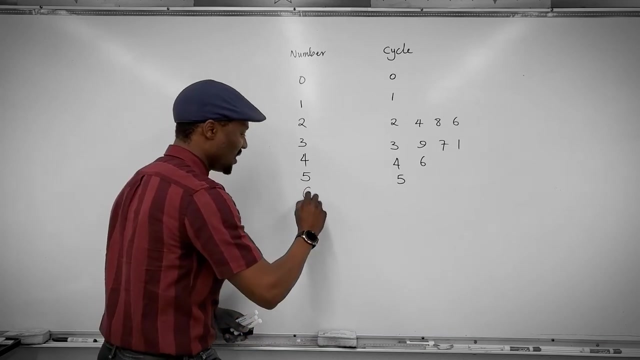 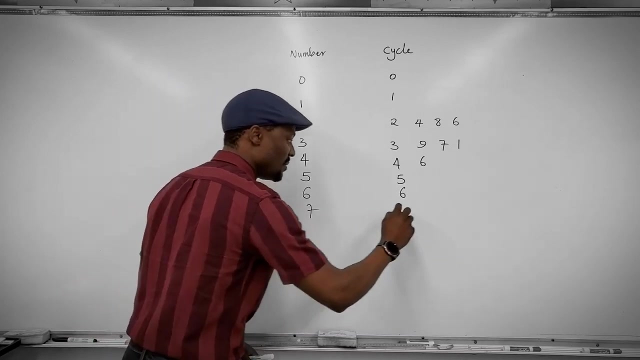 and six. the fifth number is five. well, that's the sixth number. come on, do your math, or do your math. that's gonna be five, and that to be five all the time never changes: constant six, seven, it's gonna be seven, and then a nine, and then 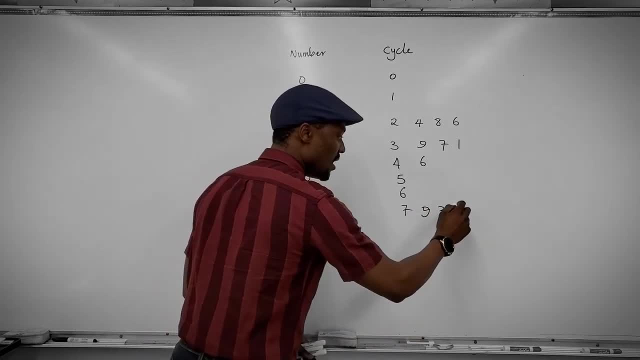 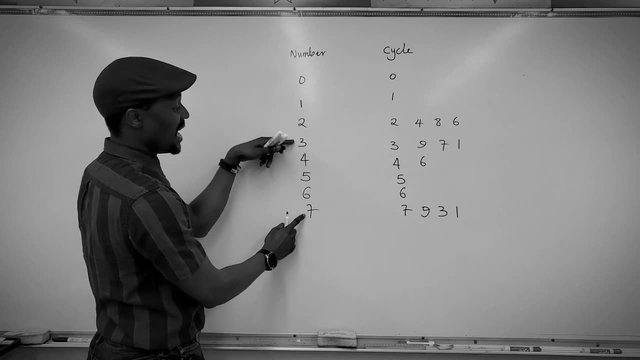 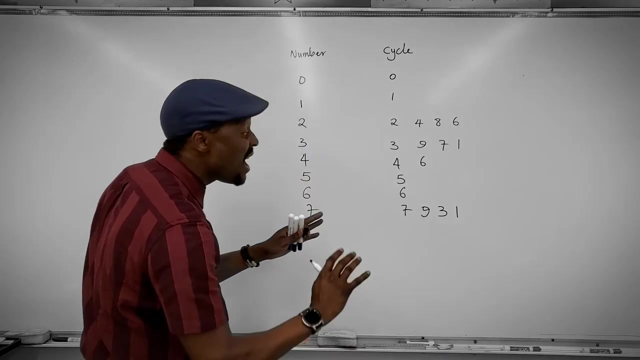 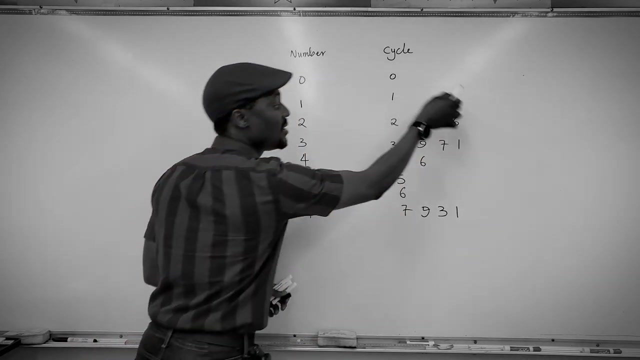 three and then one. you see anything like this. someone needs to be able to explain why this and this behave the same way. I don't get it. it might be a secret. they behave the same way, but in opposite direction. you see, seven, nine three, one seven, nine three, one, seven, nine three, one, seven. you. 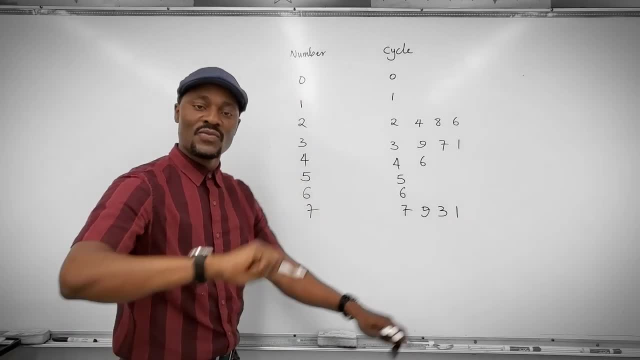 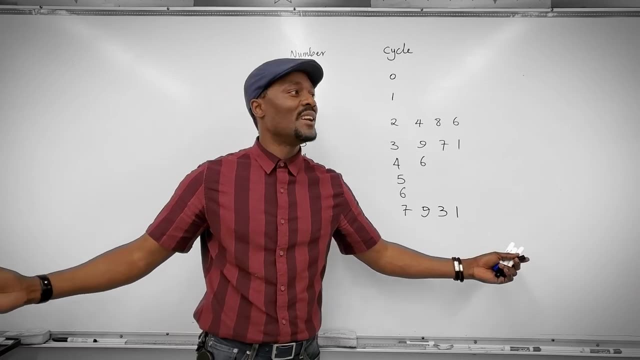 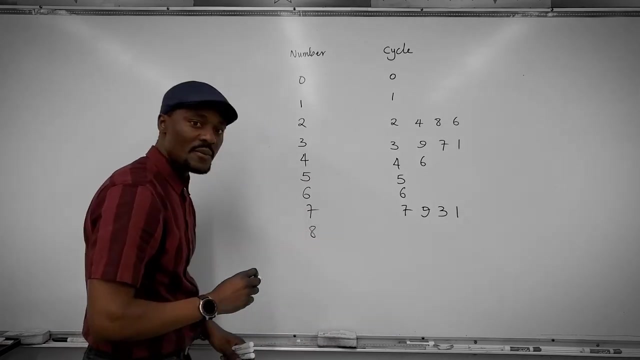 see that seven, nine, three, this one, this one is going in the clockwise direction. this is going in the counterclockwise direction. somebody tell me the mystery. okay, let's go to number eight for eight. it's gonna start with an eight, then it goes into a four. 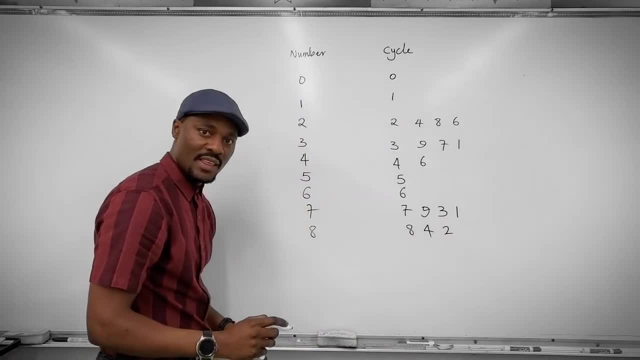 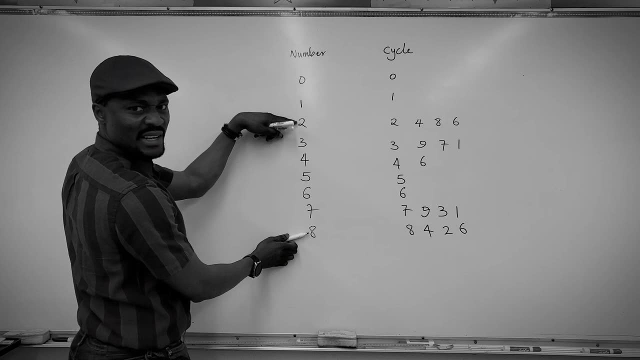 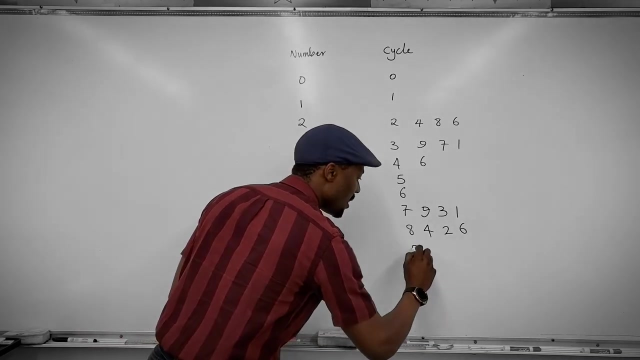 and then it goes into a two and then it goes back to a six. can you tell me why these to behave the same way? I don't get it. I don't get it. nine is the last digit. we start with nine, you end with one and it goes back to nine. 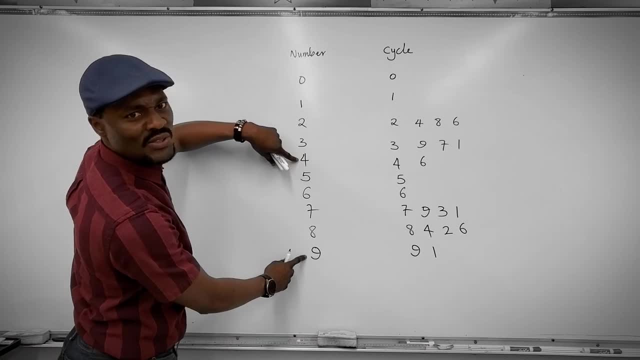 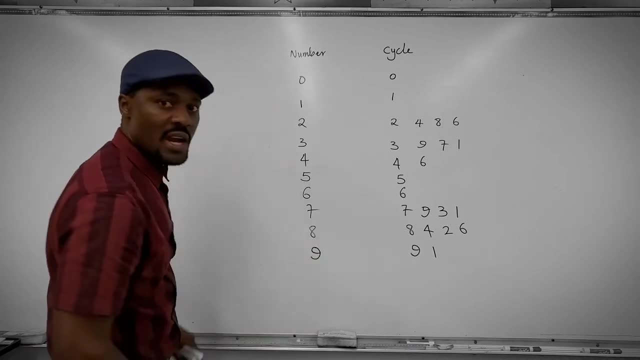 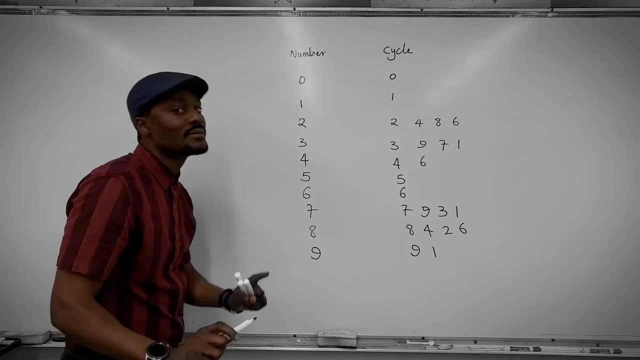 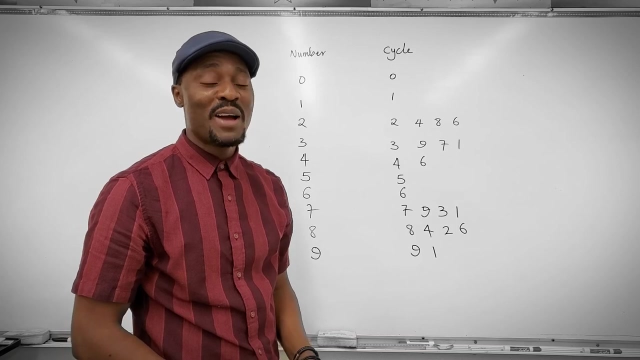 Ah, do you see these two? Well, I know the secret to this. I know something about them. it's special. It's because they are the only two perfect squares. apart from this, Thanks for watching my video. Please let me know what comments you have for me. 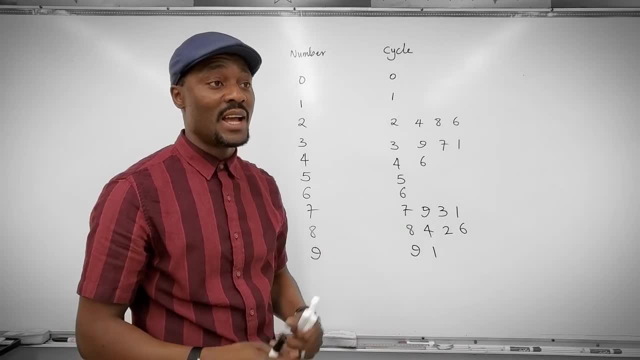 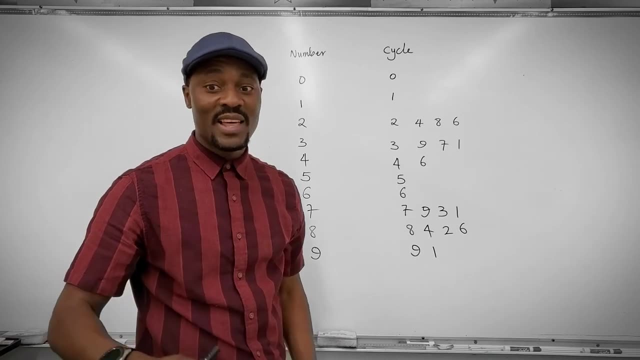 I would like to improve my videos. This is my second video and I would really like to improve. I didn't edit this video. I don't know how to edit. I'm still working on that. If I get any kind of help, any kind of advice I can get.